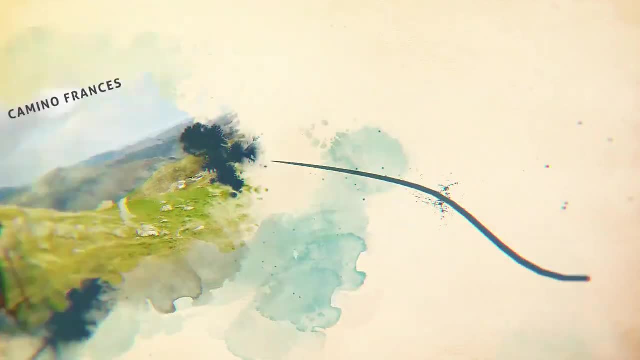 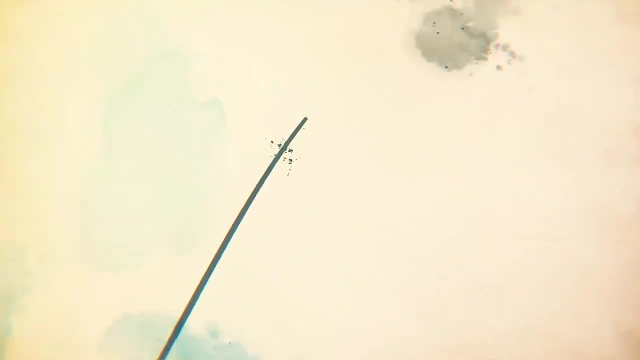 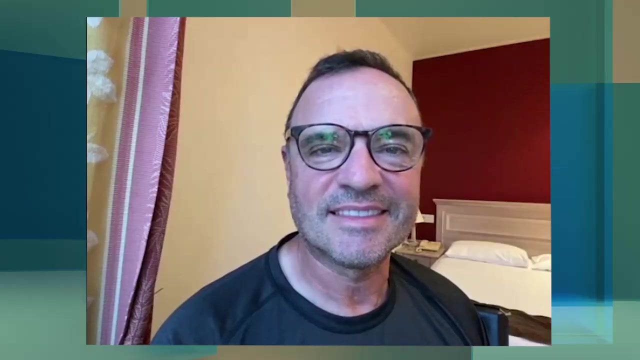 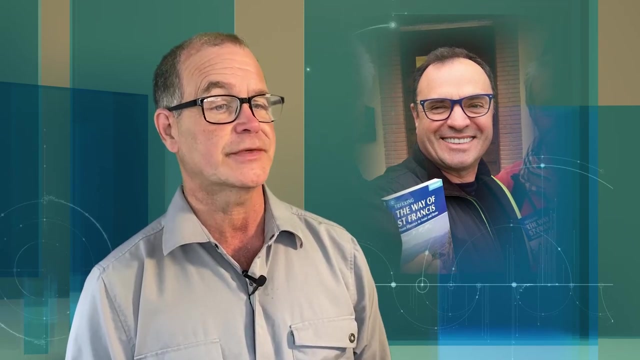 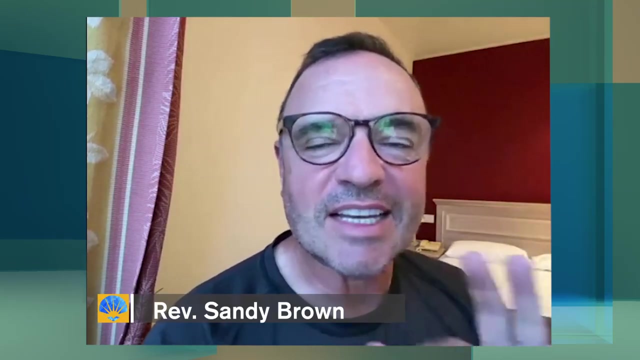 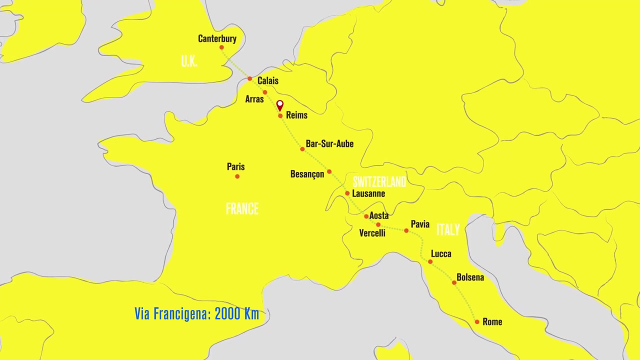 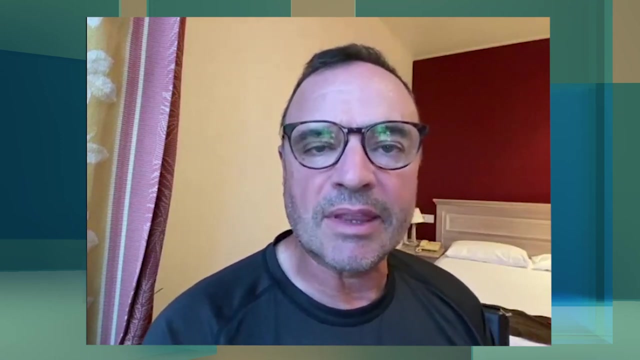 I'm pleased to introduce Sandy Brown, an author, a reverend and an avid walker, and so we're pleased to have you here and right now. where are you, and can you tell people about yourself a bit? Hi, Jim, I'm here in Reims, France, and if you don't, if that doesn't sound familiar to you, it's spelled R-E-I-M-S, and, among other things, it has one of the most beautiful cathedrals here in France, and I'm in the process of writing the first volume of the Via Francigena series. 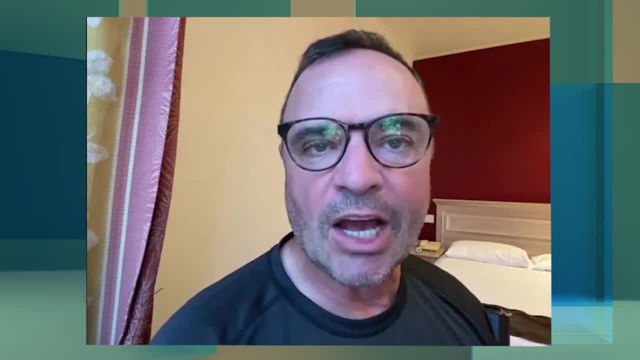 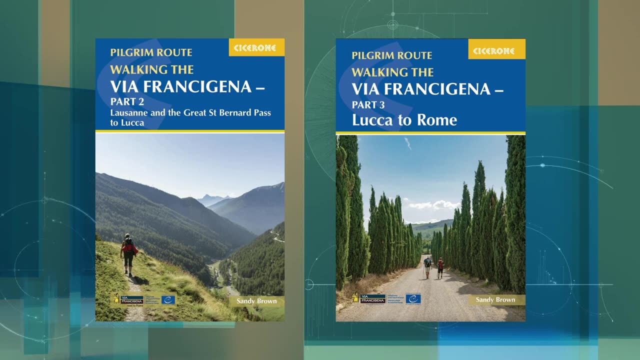 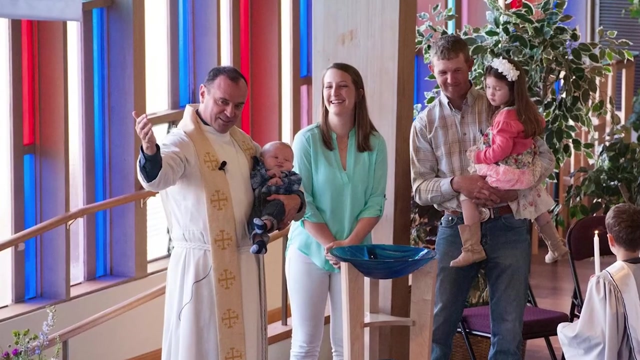 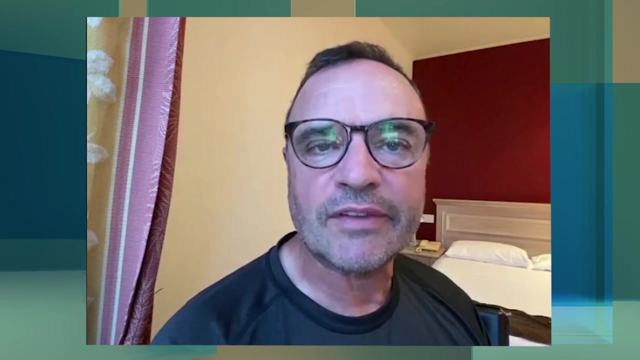 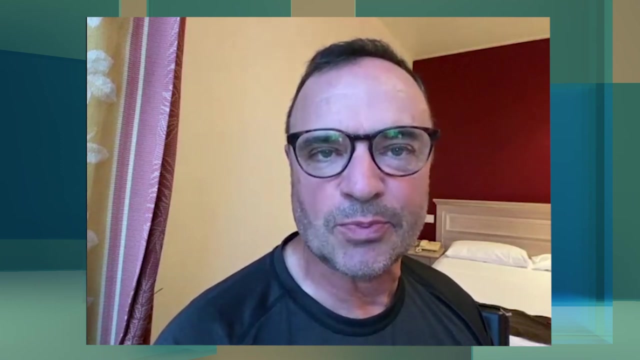 I've already completed volume two and three. Now I'm doing the part of the Via Francigena between Canterbury and Lausanne. So, as you said, I'm a pastor, retired United Methodist minister in Canada- that would be part of the United Church- and I have been walking every vacation since about 2008, after being inspired by Paulo Coelho's book. 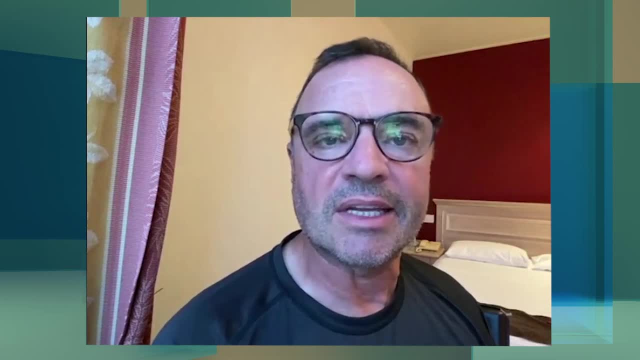 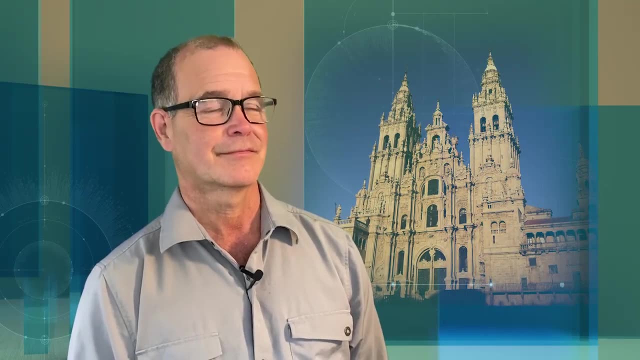 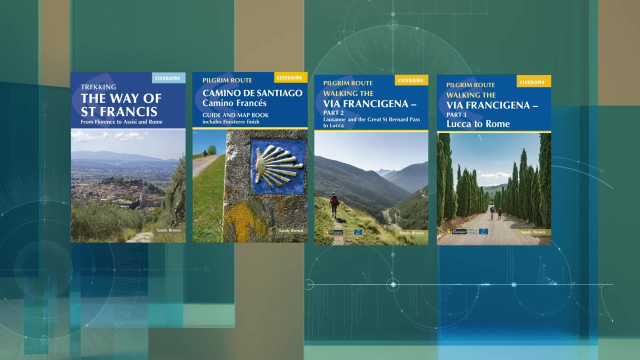 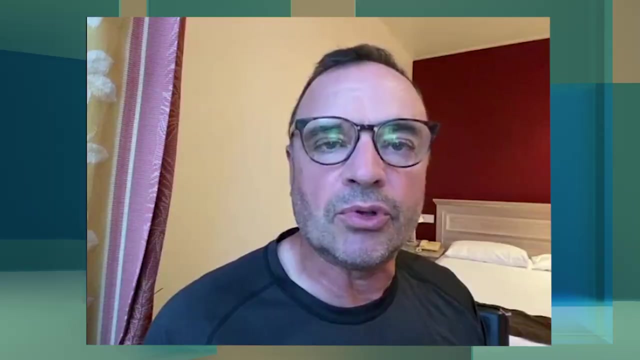 the pilgrimage, I walked the Camino de Santiago and since then I've walked about 12,000 kilometers in Spain, France, Switzerland and Italy. I started writing guidebooks in 2014 and I'm on my fifth and sixth guidebooks right now, and I really love helping people to discover these great pilgrimage walks. 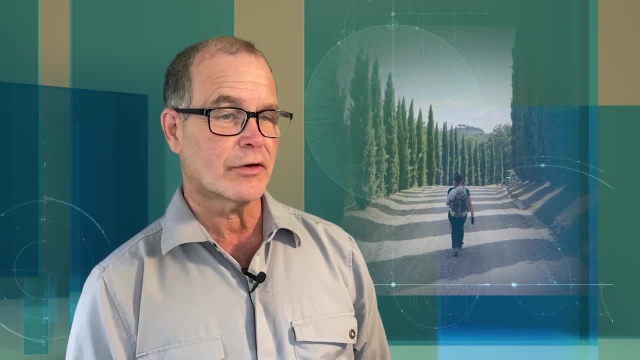 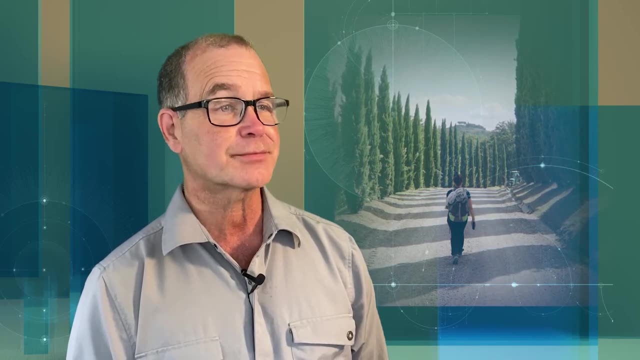 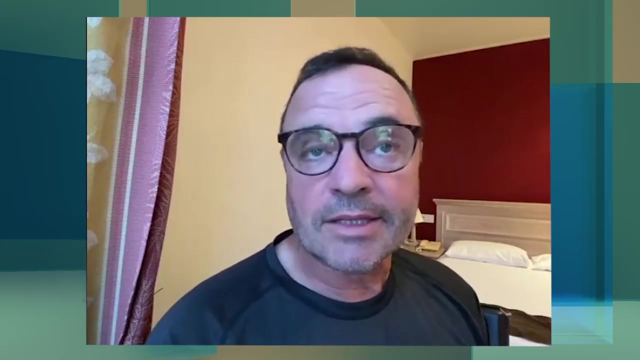 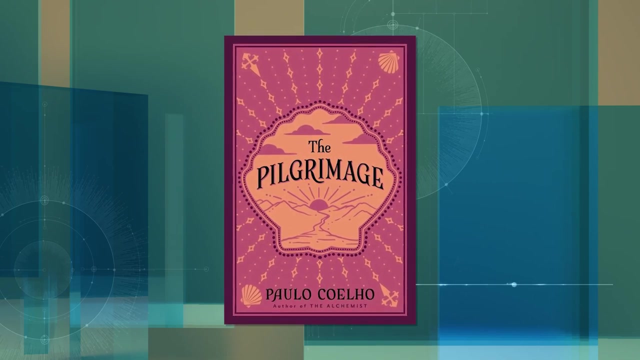 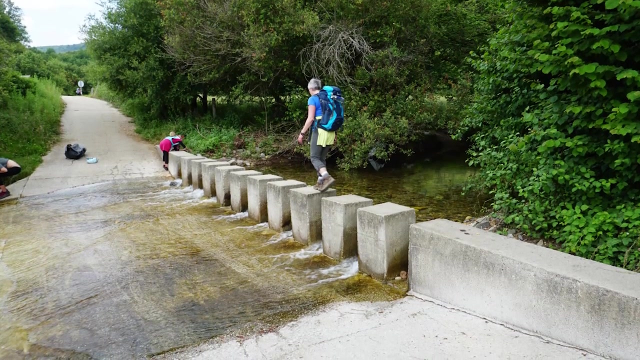 I can't believe, Eric Dickinson, when we've done six walks, When I saw how many walks and how many kilometers you were. you are truly inspirational and I'm just trying to figure out what inspired you to walk in the first place. Well, as I alluded to, I read the Pilgrimage by Paulo Coelho and what fascinated me about that was the idea of walking in Spain, because my heart was: if you want to walk in a pilgrimage to the 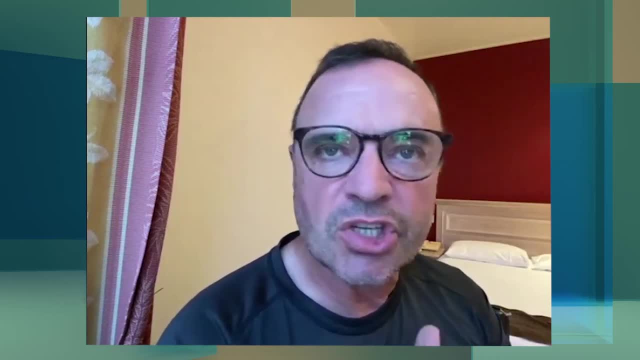 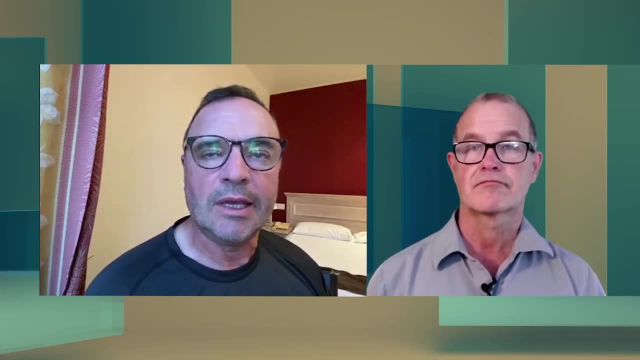 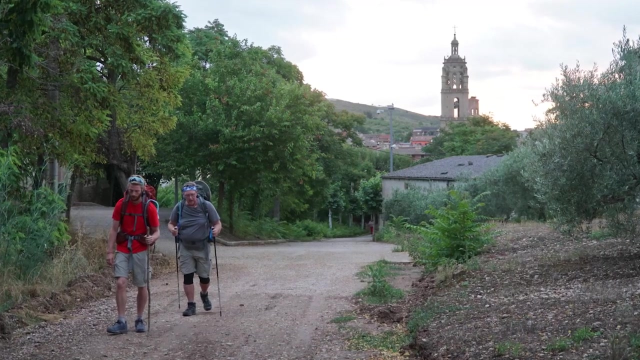 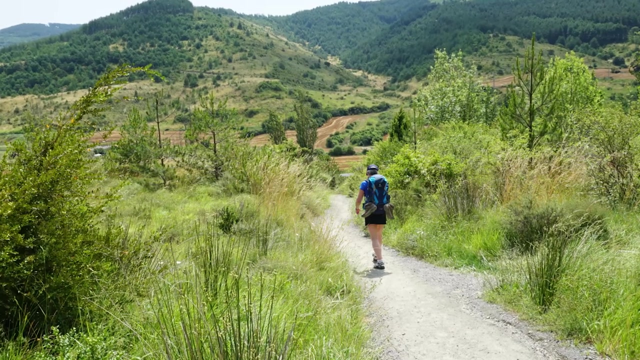 family has some roots in Spain that we're continually trying to uncover, and I thought what better way to connect with the country where some of my ancestors came from than to walk? and it sounded like a great adventure, and so I read the book The Pilgrimage in 1992. but I didn't get to the Camino de Santiago until 2008. so everybody that's ever walked the Camino probably has a story like that, where you set your goal but it takes some years to be able to arrange your life so that you can meet that goal. in my case it was 16 years, but once I did it once. 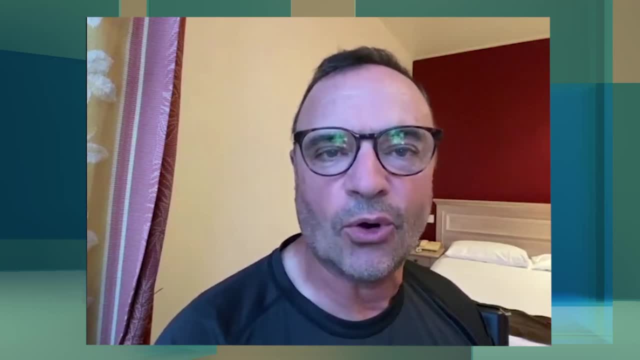 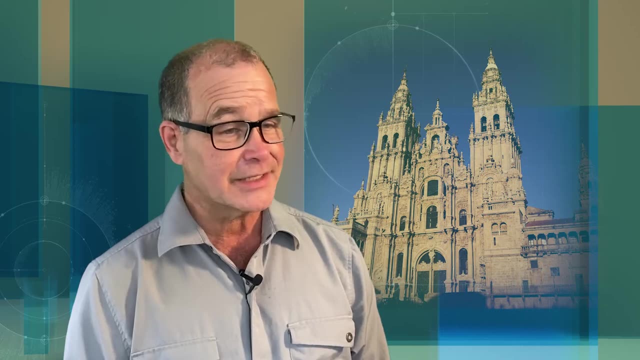 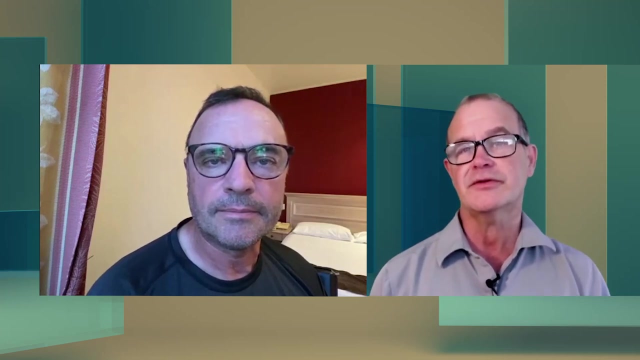 I was hooked and I wanted to go back and back over and over again. well, you truly inspire me, you're amazing and you've also taken the time to write books, and that many people have done blogs but you've done books. can you talk about the names of the books? 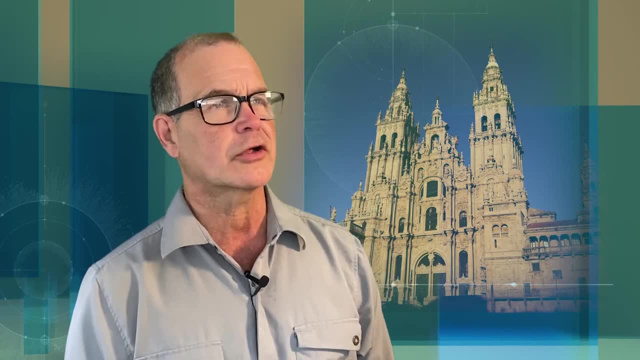 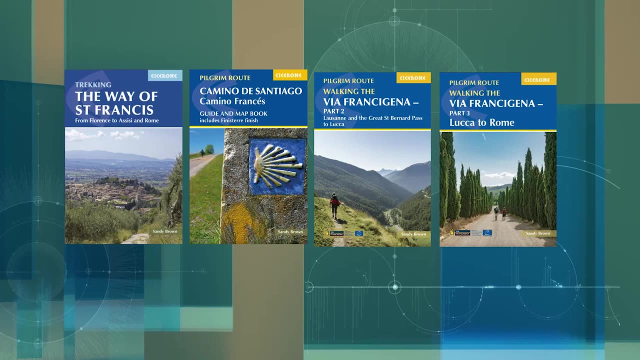 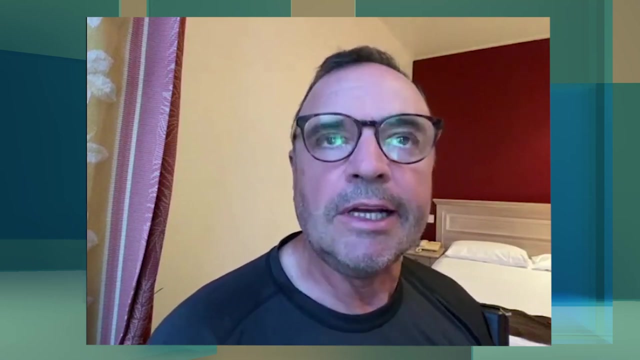 and can you talk a little bit about what your books are all about? sure, my books are all guidebooks and I work with Cicerone Press, which is one of the largest English language guidebook books makers for outdoors. and so what happened was I was walking the Camino del Norte. 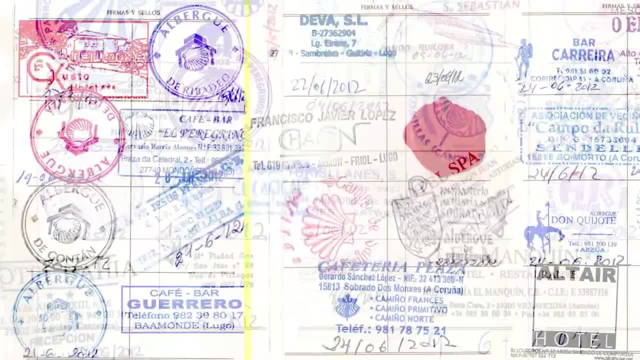 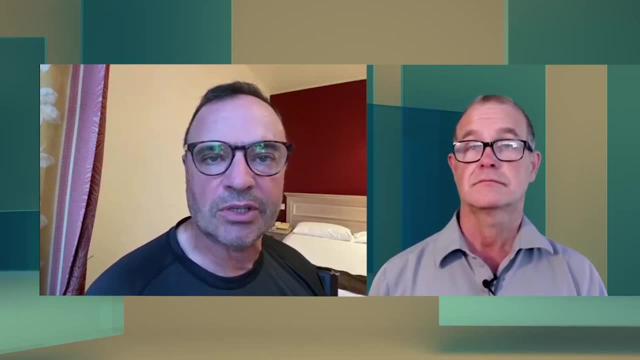 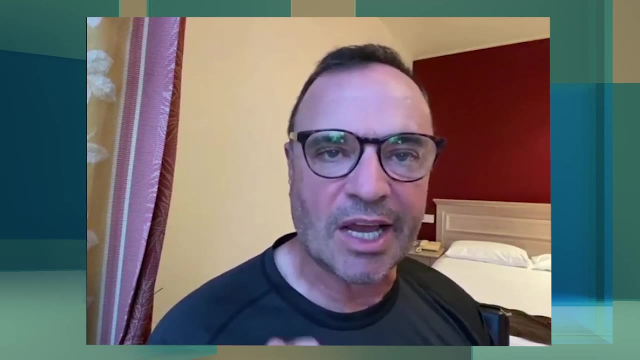 and I realized it was not a very good- or actually at the time there was no English language guidebook. so I picked up the French language guidebook to the Del Norte and I used a website that had the Spanish language guidebook and I put those two together and I thought, wow, this really. 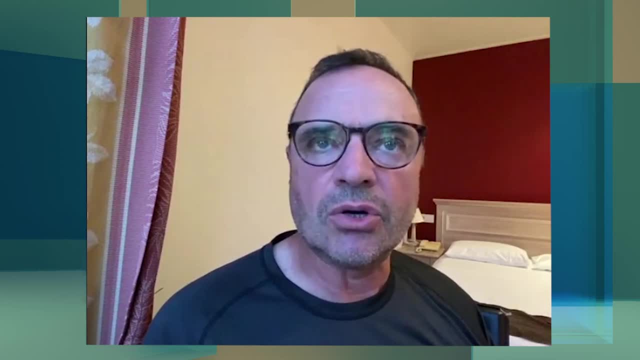 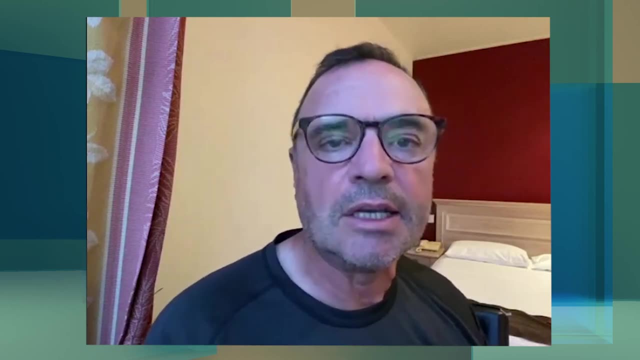 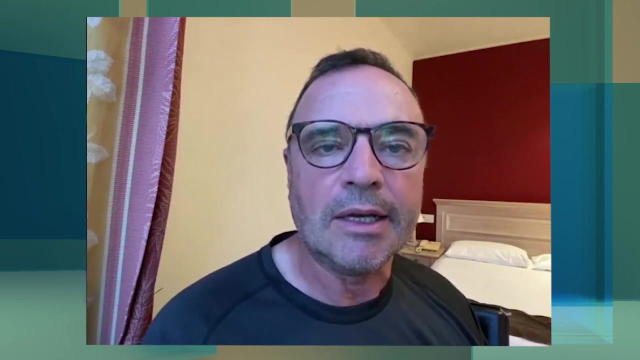 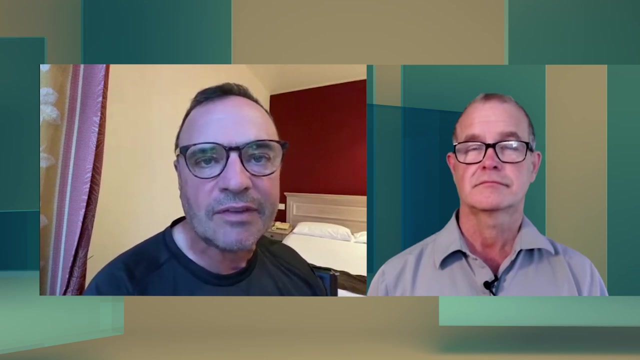 needs a guidebook, and so I began to look around for who would be willing to publish that. I contacted Cicerone Press. they said: oh, as it turns out, we actually already have a guidebook in the works for that. and the next year I walked the way of Saint Francis in Italy. I loved it, and so then I 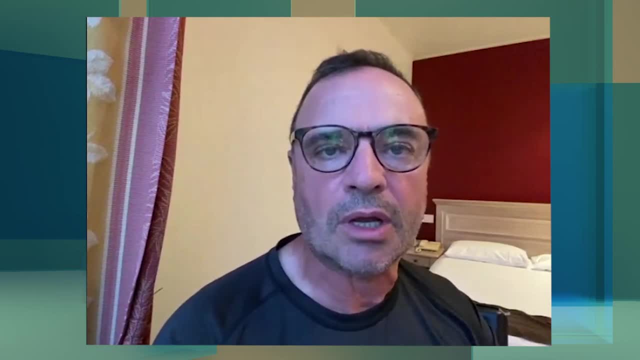 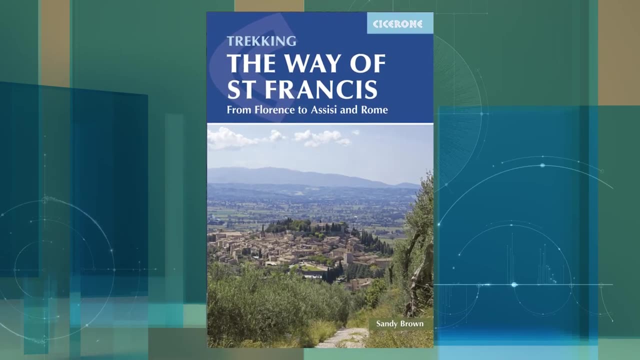 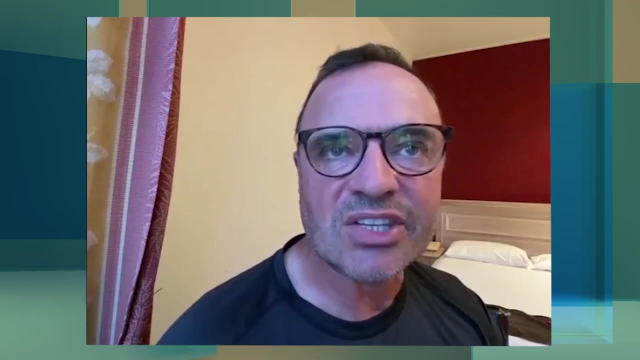 proposed to Cicerone Press that I would publish a guidebook for the Del Norte and I said I would write a guidebook on that walk, which I did. that was my first book. they asked me to write the new Cicerone guidebook on the Camino Frances, which was published in 2020, and I asked them if I'm going to. 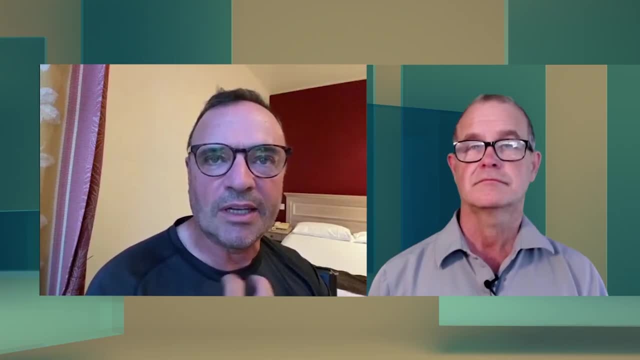 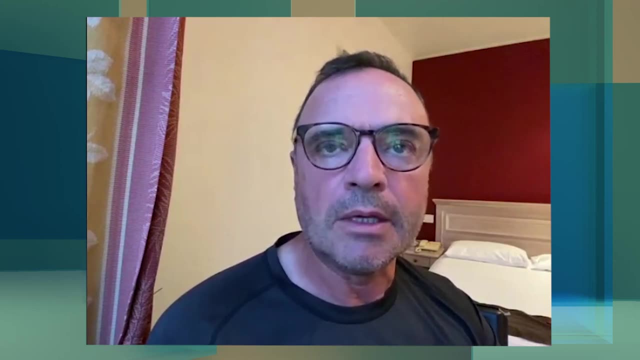 do the Frances guidebook. I'd like to do one that I would really love to see a new guidebook for, which is the Via Francigena. so we agreed that would be in 2020 and I said, okay, I'm going to do a guidebook on that. 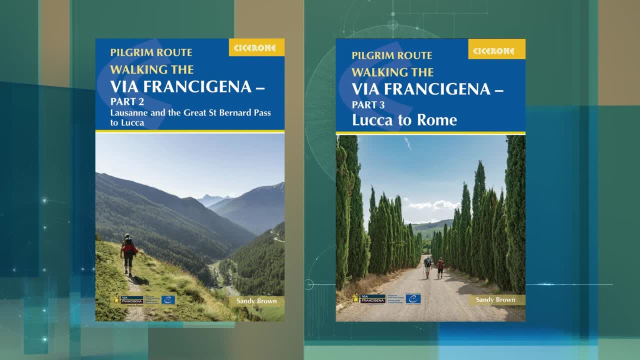 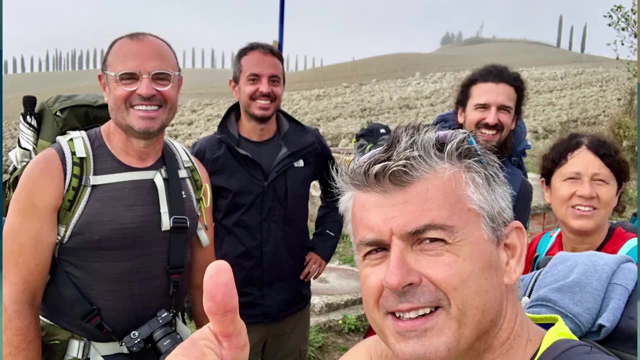 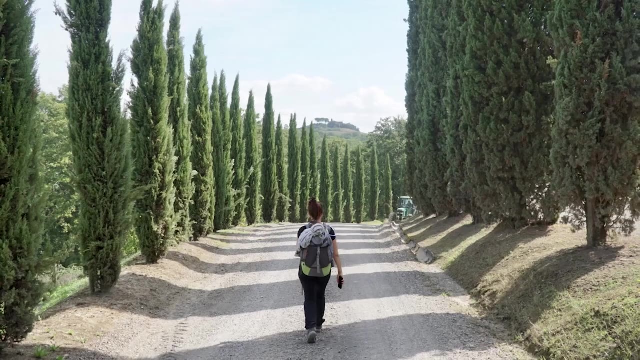 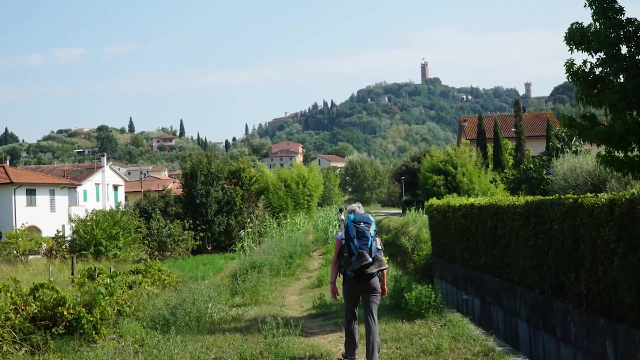 and here it is in three volumes, and that's what I've been working on since about 2017. so I got into it because I was a walker and I wanted walkers who speak english to have good guidebooks, like the French and the German and the Spanish do. so that's what got me started. 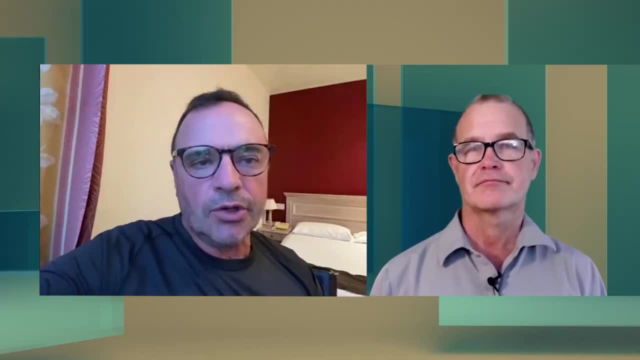 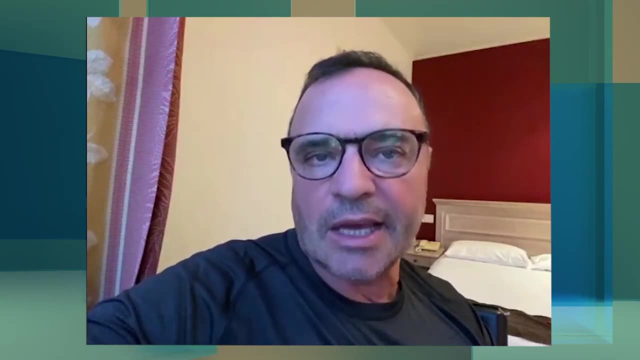 so and how would that differ from other guidebooks? We are instituting a new pilgrimage guidebook format and the Del Norte book is not in that format yet. The first of the new series is the Camino Frances book and that was published in 2020.. 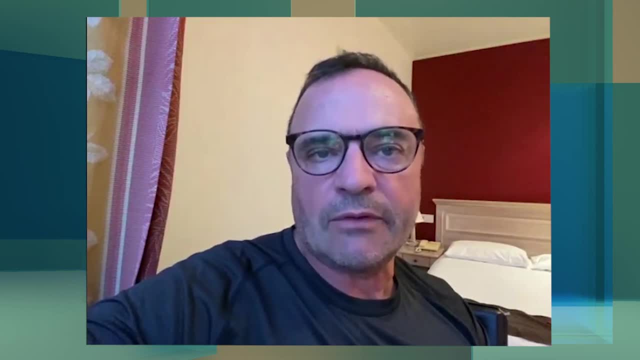 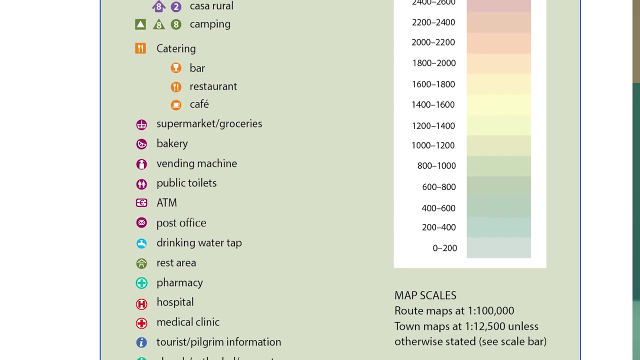 So everything after 2020 will be in the same format And the most important things are, first of all, on accommodations. So every accommodation will have 22 different fields of information that will help pilgrims be able to decide if they want to stay at that particular accommodation. 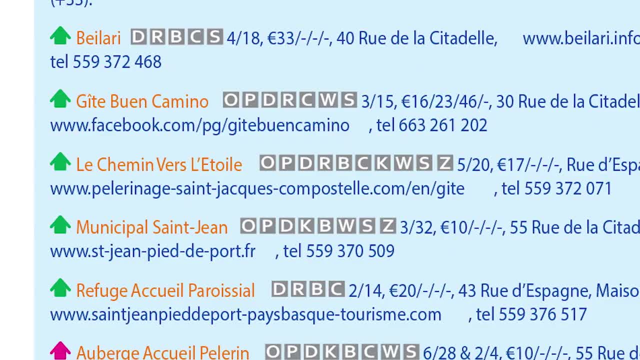 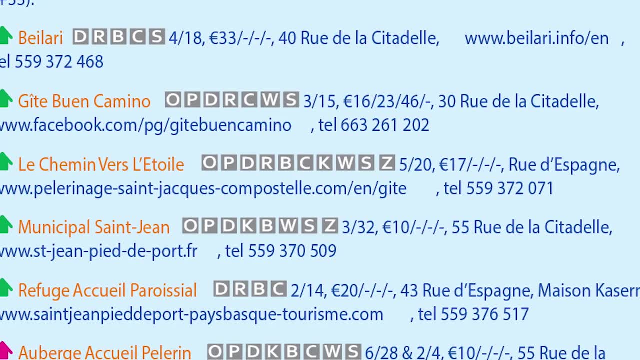 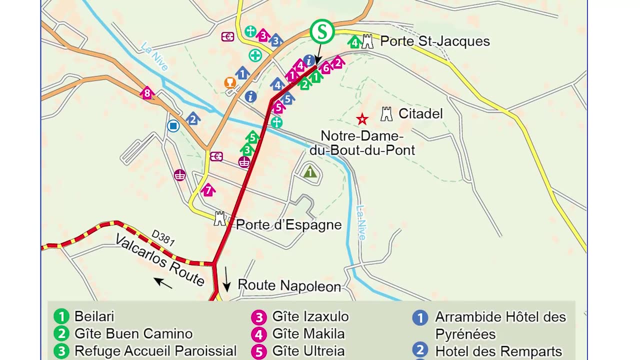 So, for instance, we could tell you if you could use a credit card. we'll tell you if there is a disability accessibility, if there's a communal dinner, if breakfast is served, if there is dormitory, Dormitory, sleeping or private rooms and many other things like that. 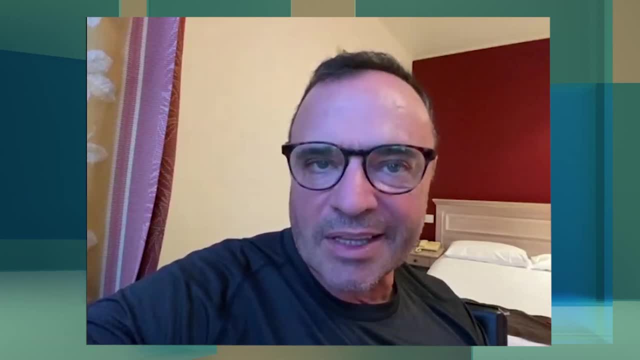 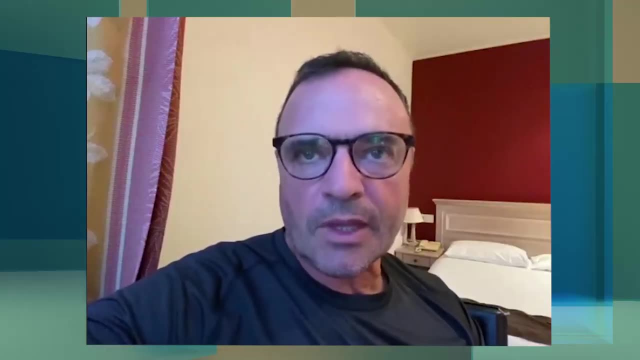 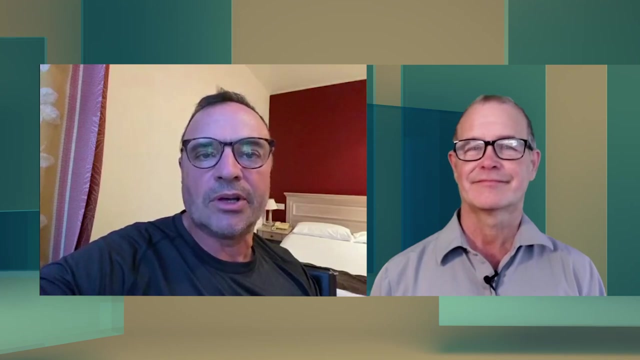 And so that's one example of how we're going the next mile And also we're making sure that our maps are to scale. So some of the most famous guidebooks out there don't use actual to scale maps. They're drawings or representations of what the route is. 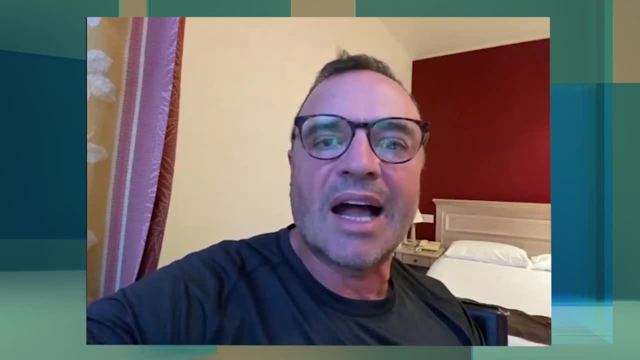 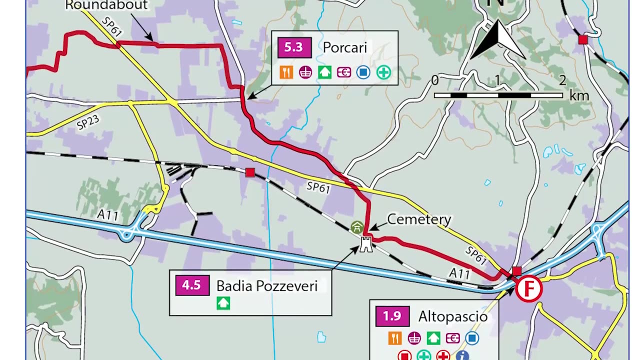 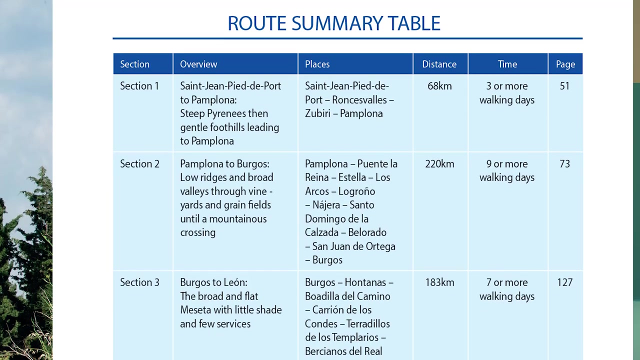 And at Cicerone we found We felt that it's important to have the actual map And, plus, our maps always face north up so you always know where you're at in comparison to the cardinal directions. Then we always have an appendix at the end, which is a table that shows you distances. 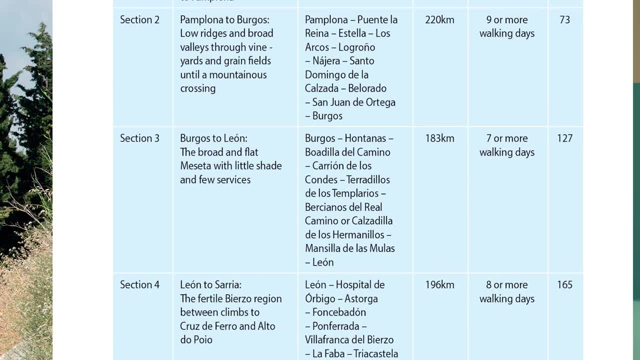 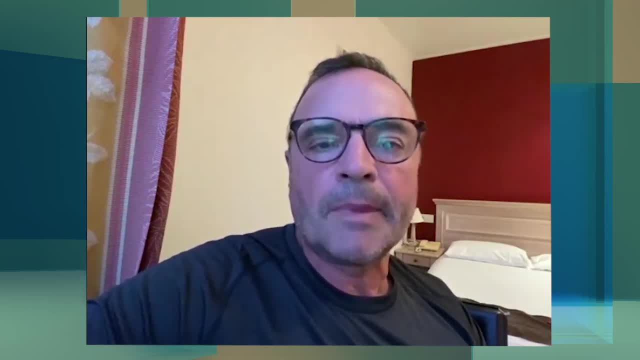 between places where there's accommodations, so you don't end up at somebody else's stage end. all of the accommodations are booked. Instead, you can design your own stages very easily with that. We call it Appendix A. So those are just some of the ways in which we're changing and 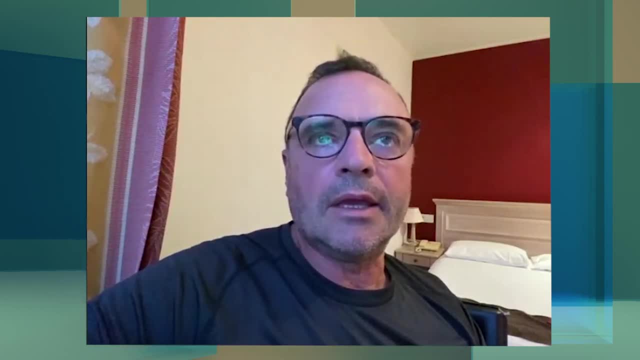 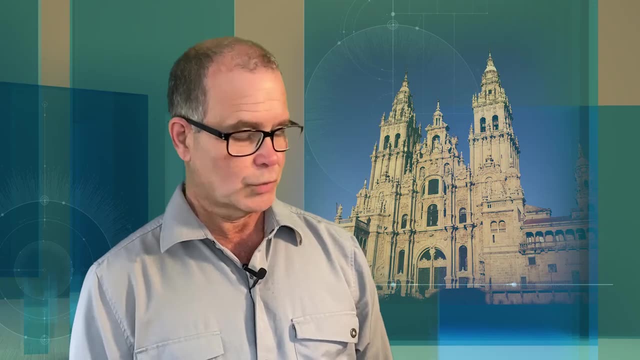 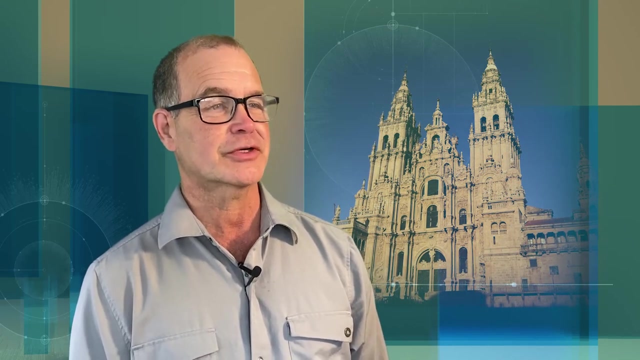 in my opinion, updating the idea of a Pilgrim Ranch guidebook and really making it state-of-the-art and next generation. Well, I can tell you, as a walker who used the German book and the English language book The First Pilgrimage where we were looking for some material from 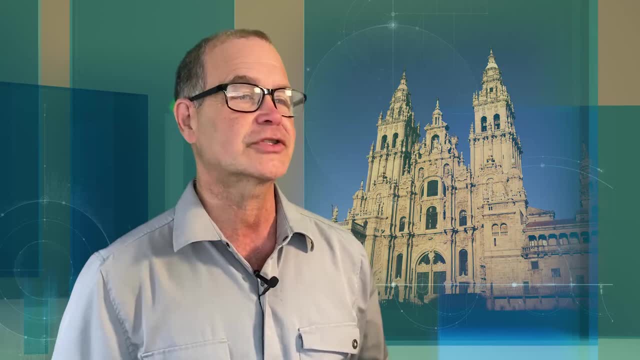 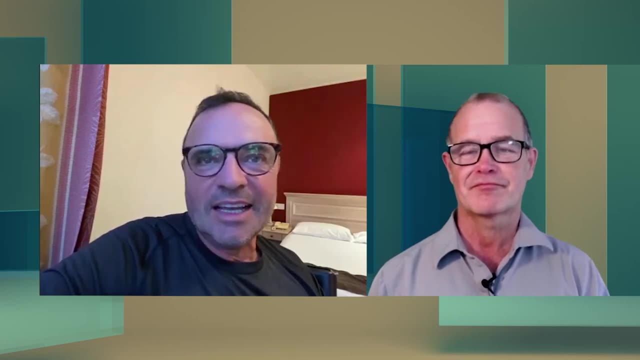 one place and some material from the others. I appreciate the way you're approaching your guidebooks. Good, good, Thank you. One thing I like about the German guidebooks is that they will tell you where a laundromat is, And at one point I thought that was just. 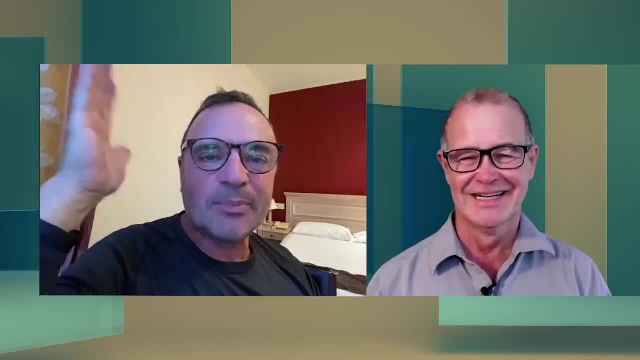 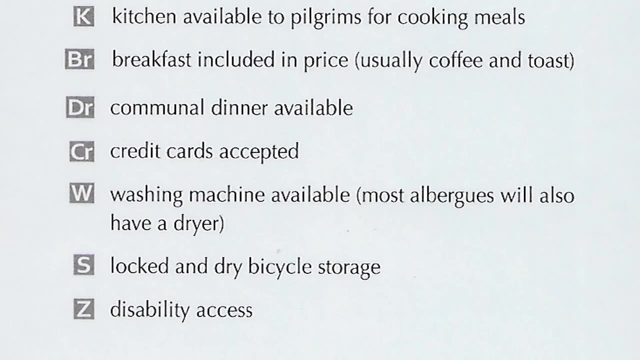 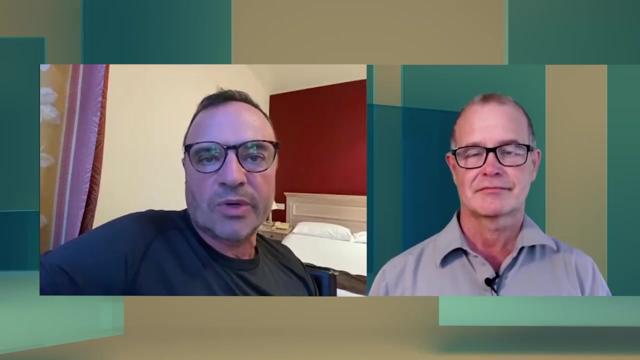 too much detail, But no, it's actually something you can really use, So we included that in the data of ours. Nowadays, albergues oftentimes have washing machines themselves, So we list that among the 22 different data fields for each albergue, and it was inspired by the Germans. 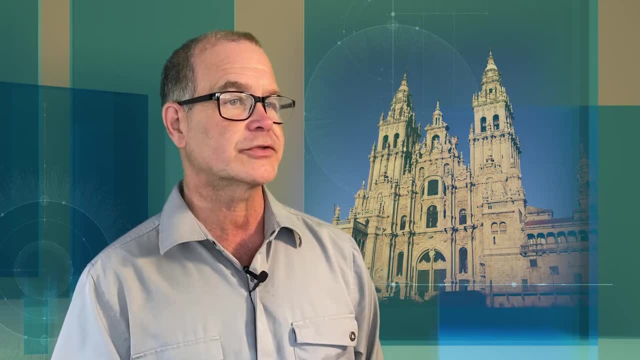 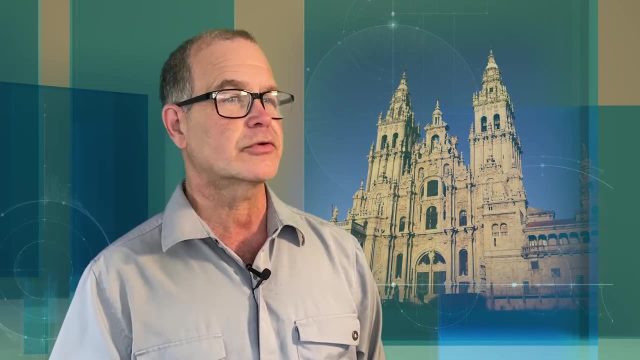 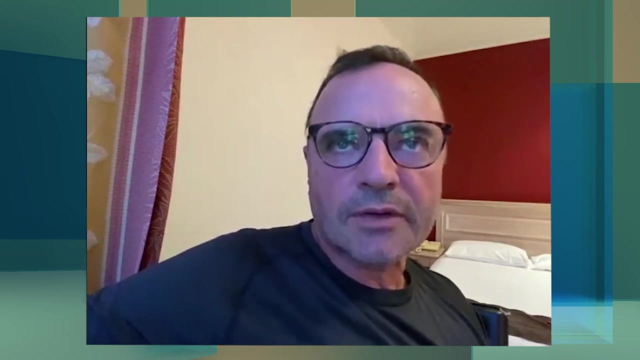 Thank you. How would you approach the walk? You started the first walk in 2008, and you approached it. You've done multiple, multiple walks. How has your approach to the walk changed over all those years? Yeah Well, first of all, I would say that there is an aspect of my preparations that is different now. So the first time I walked, I think by about the end of the second week, I had about 12 big blisters on my feet And it took me a few years to find a system that works for me And I moved from hiking shoes. 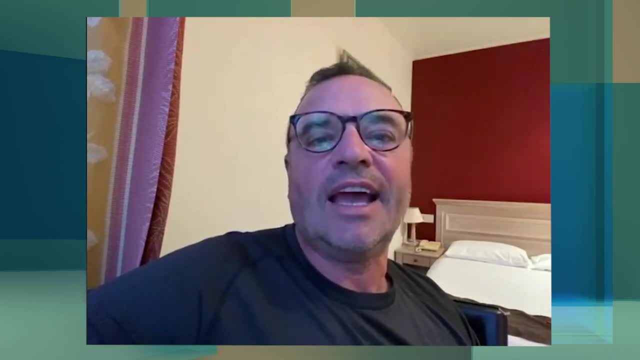 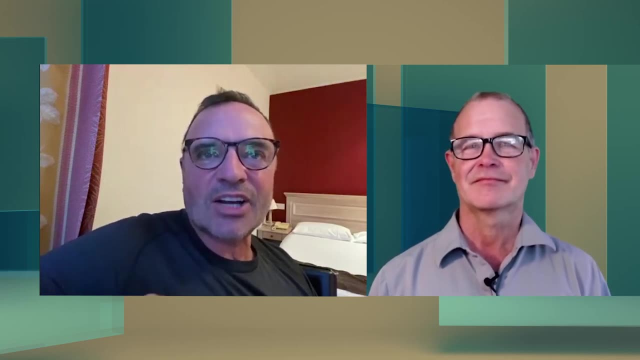 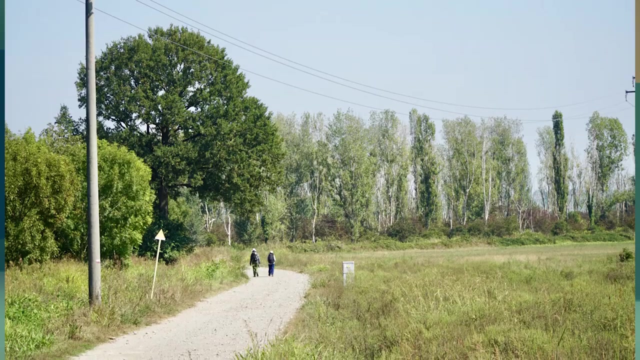 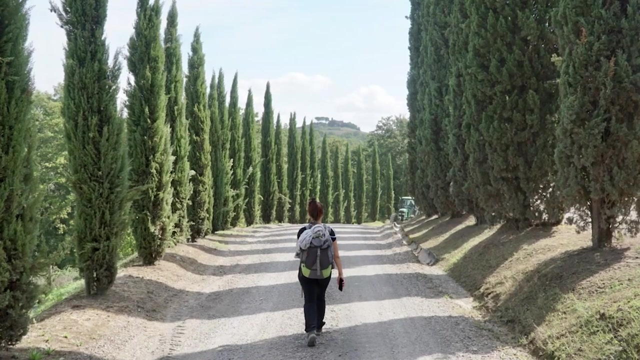 to hiking boots, to hiking sandals and now to trail runners, as you know, what I put on my feet And that's actually, I think that shows, in a way, the evolution of my own thinking. I've changed from seeing it as a hike to seeing a pilgrimage as as something of an ordeal that I have to. 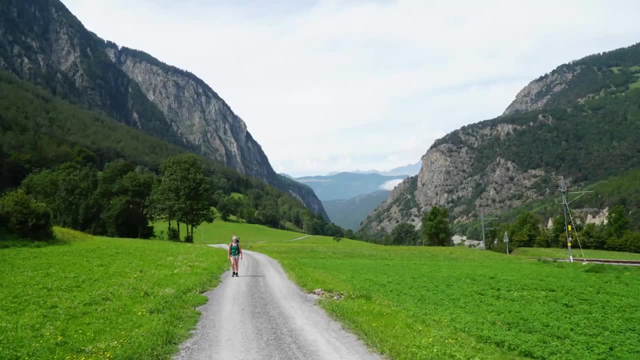 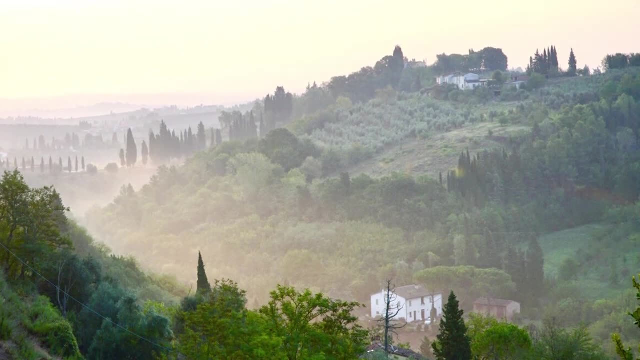 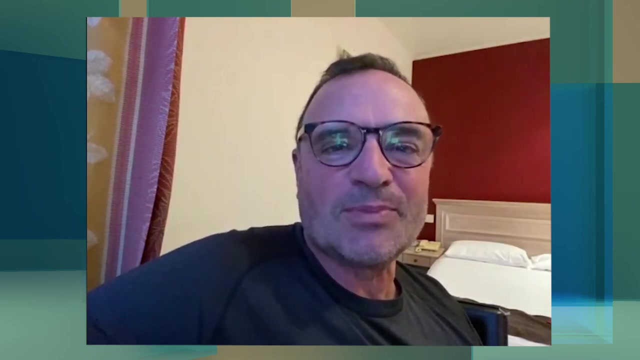 master for my own well-being, So I know what I need. I know that after three or four days, if it's been hot, I need to go to the pharmacy and get some magnesium potassium so that I can recoup those minerals that I've lost. 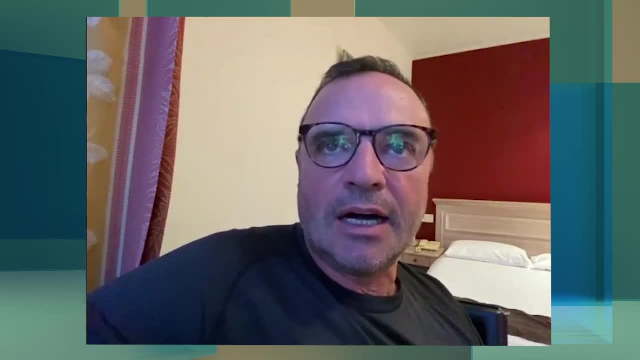 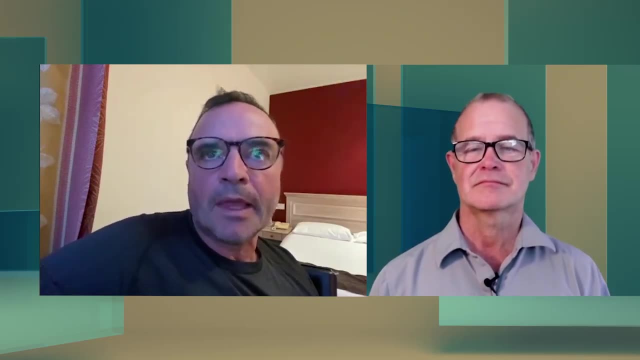 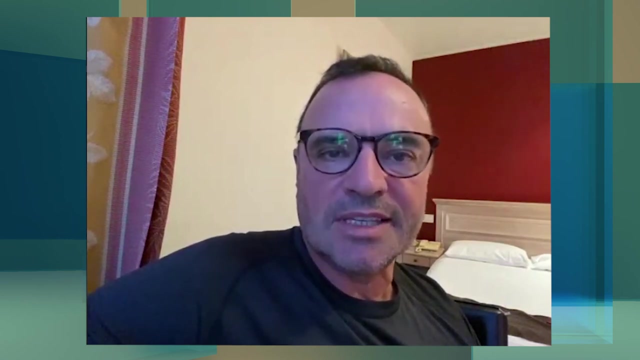 So, in the preparations and the way in which I'm dealing with my body, those are things I'm better at In terms of what happens to me on the walk. I'm used to this now, And so I remember sitting on the Camino Francis at the heights above Lagronio and Viana. 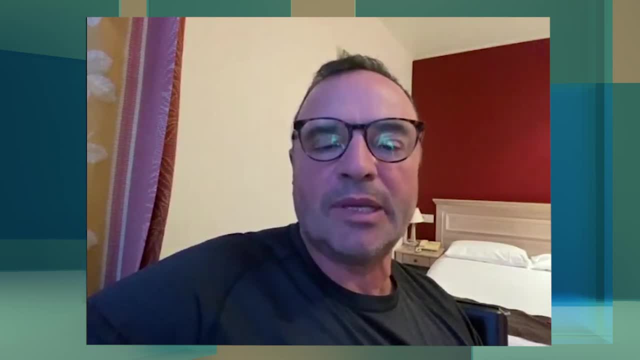 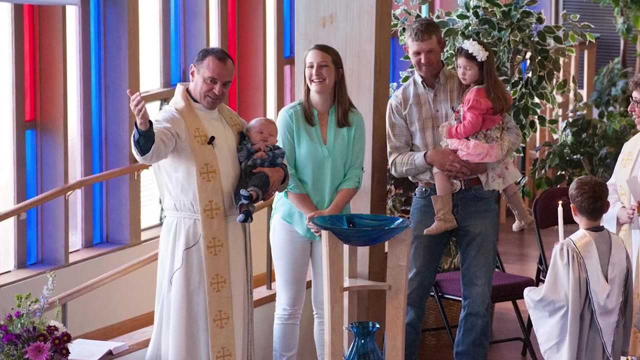 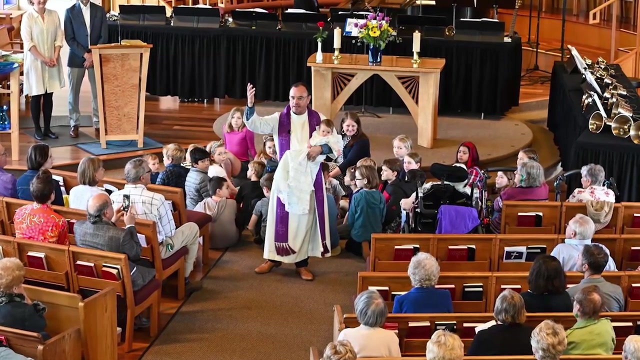 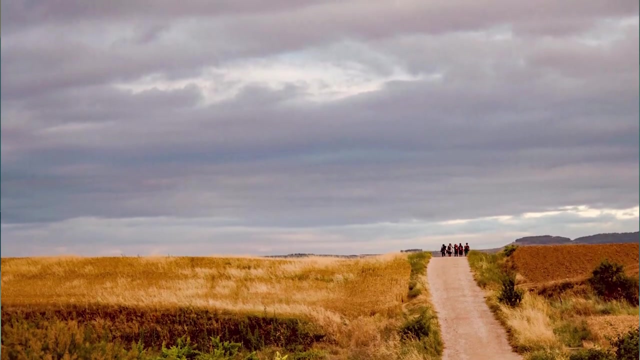 and writing my journal about what it was like to be by myself and it was unusual. i mean, a pastor is oftentimes with people and very much in a communal arrangement, but i was experiencing solitude and i had to learn how to deal with that. on the front says solitude is unusual, but on the del norte or the 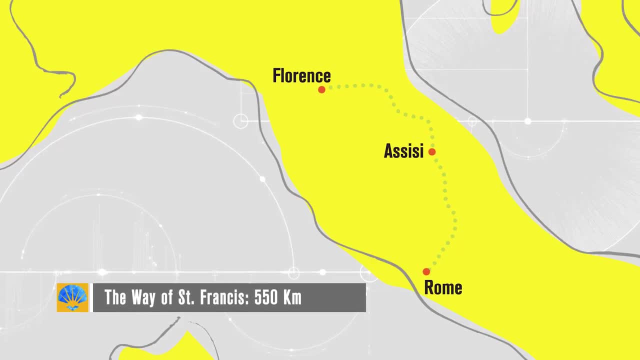 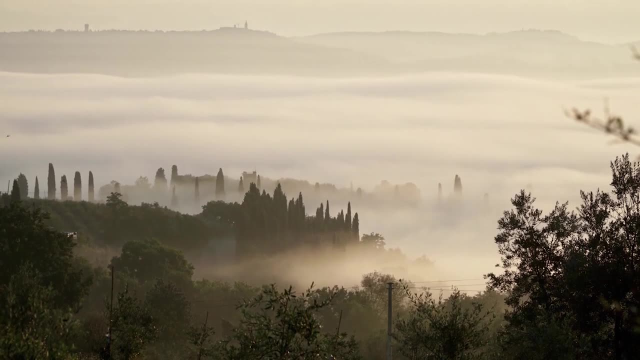 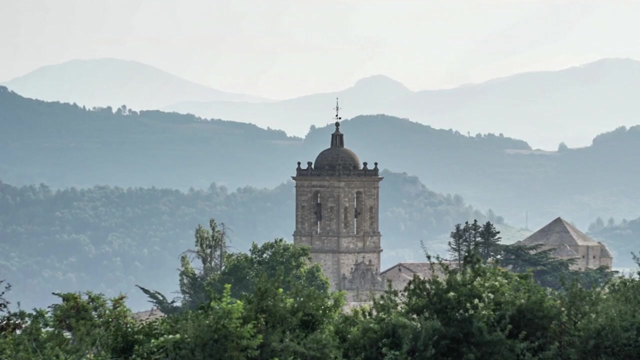 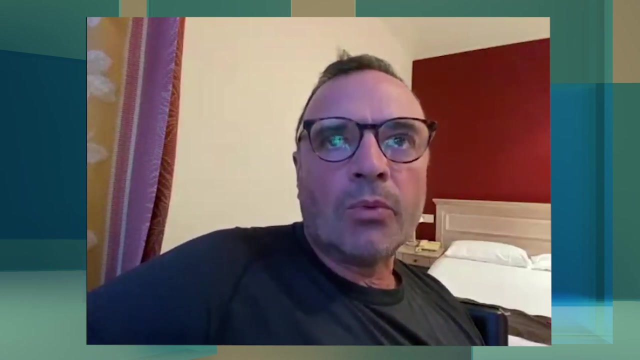 san embrace or the via francis, you know, or the via de francisco, solitude is routine. so even today, as i was making today, i was on a bike, i was doing three walking stages on a bike because i already covered these earlier this summer and i just wanted to refresh myself. i i stopped and i was in. 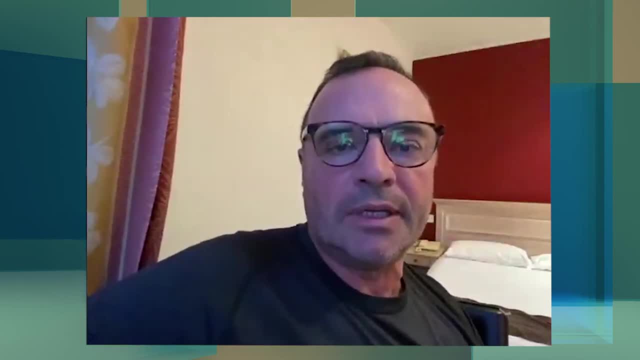 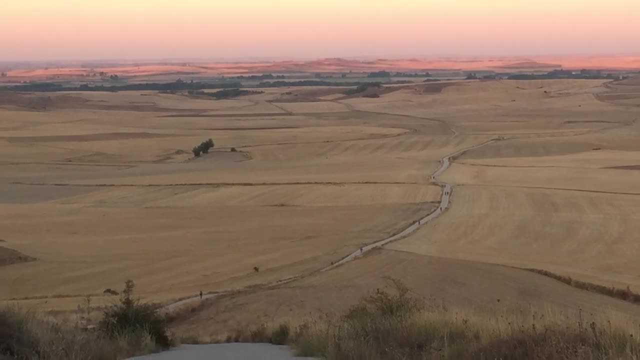 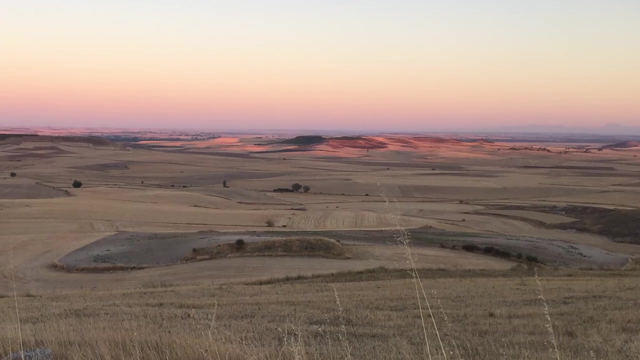 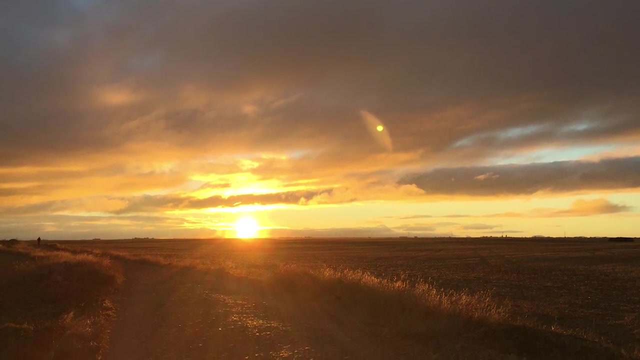 a vast field that had already been harvested and i could see for probably two or three miles in many directions, and that moment of simplicity and beauty is what makes me want to come back every single time, because it speaks to my soul. so i didn't know that that's what it was. 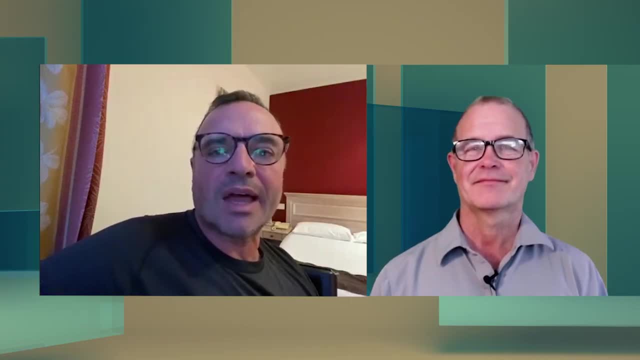 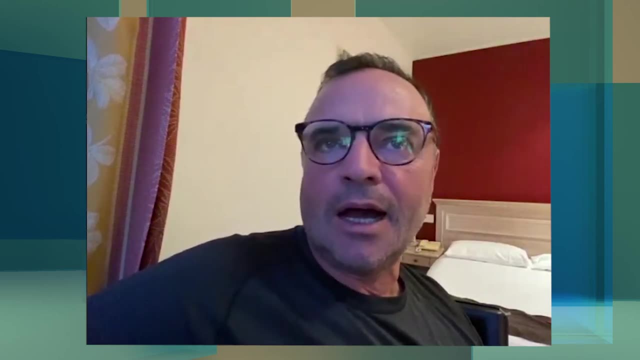 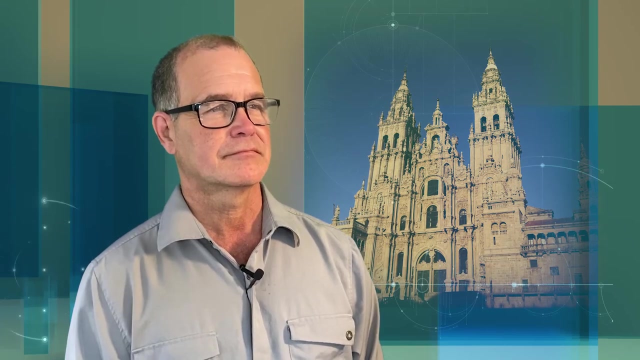 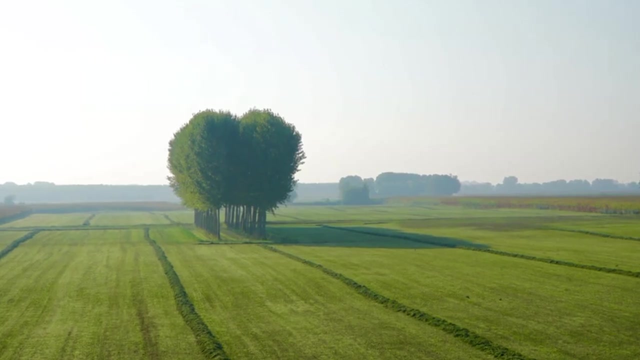 and my first camino. but i know that now and when it and when i fall into it on a stage and i find myself just in a sort of an ecstasy as i experience nature and the vastness of the world around me, it's not a discovery anymore, it's an old friend and it's a welcome. 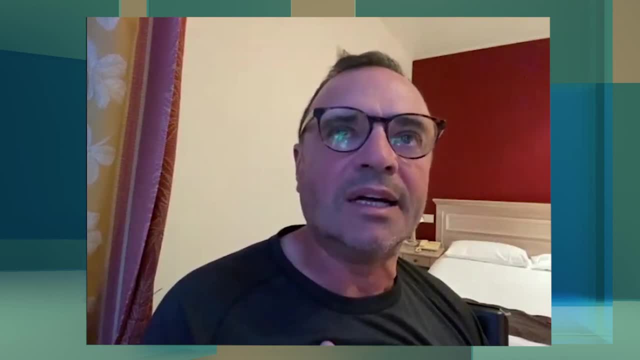 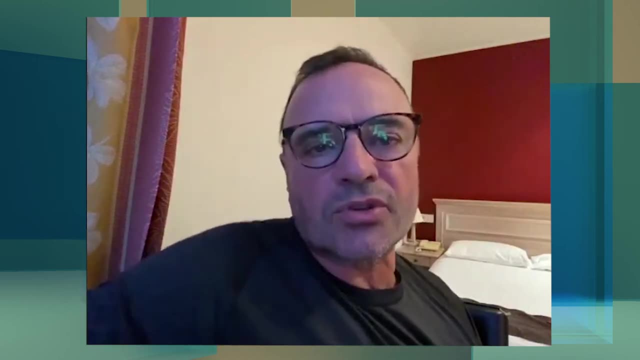 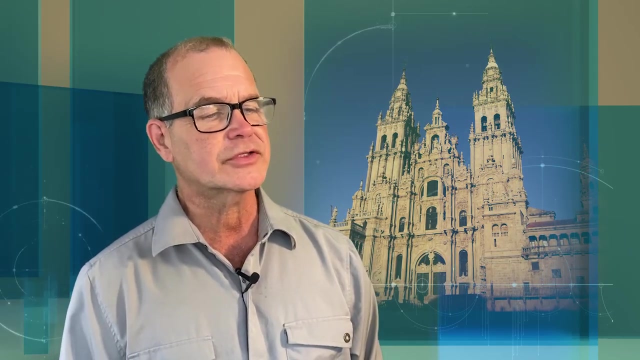 moment where i can stop and feel as though i'm being fed and nourished. so those are two ways that i'm different now, uh. so talk to us, uh, about what the average walk you walk each day and what, how you approach each day and what you expect each day. 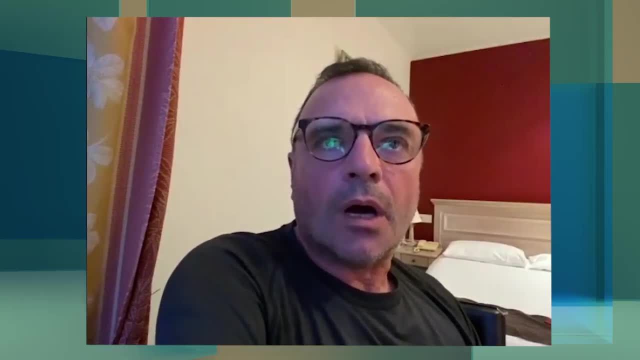 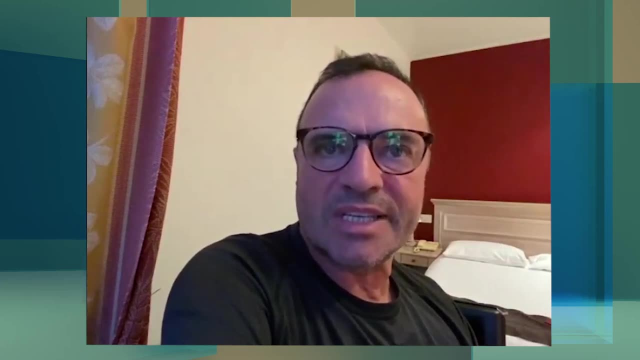 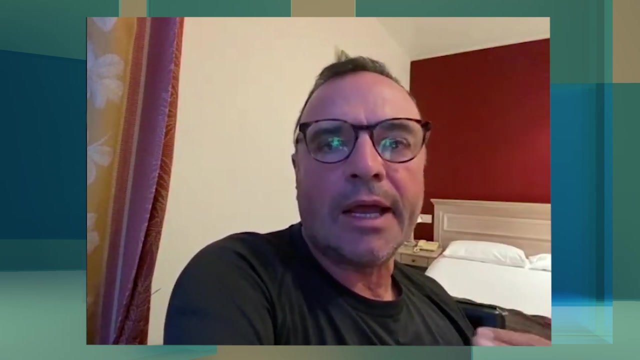 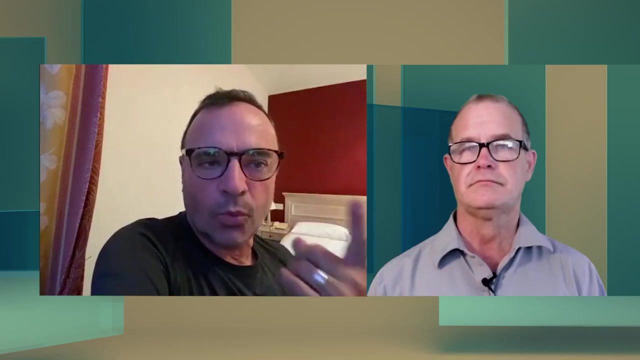 so, uh, that's different when i'm walking the camino francis or if i'm walking a less busy pilgrimage with less infrastructure. so at the start of the day now, my most important, um, my most important goals are to find water and to find food that will last me for the day. 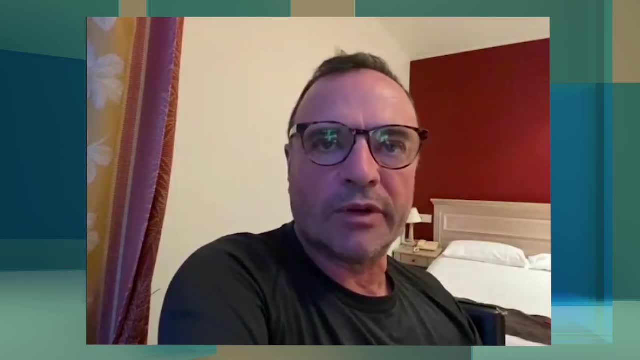 so it just happens in the francis. now, when you're in france, you may or may not come upon a village where there is a bakery or a restaurant- in fact, almost always you don't- and your next food is at the stage. and in france what's really great is that there are these bakeries, and bakeries are in. 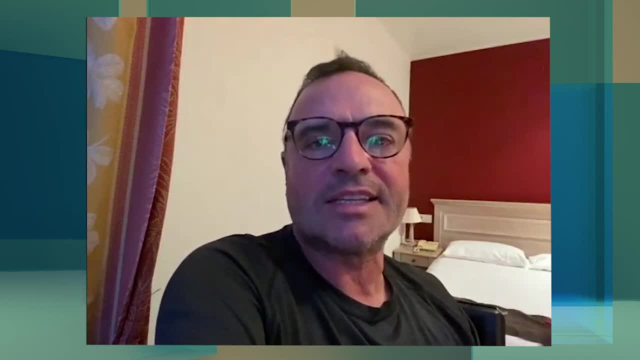 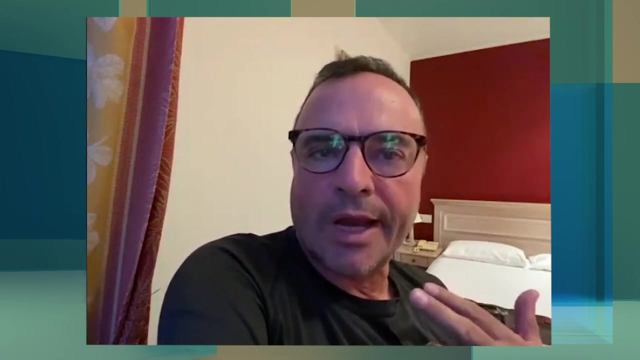 most every uh, small to medium-sized town. they make, they make. they make not just baguettes and sweet treats, but they'll also make you a sandwich. so i get my water, i get my sandwich for my lunch, so i have enough food to make it through the day. 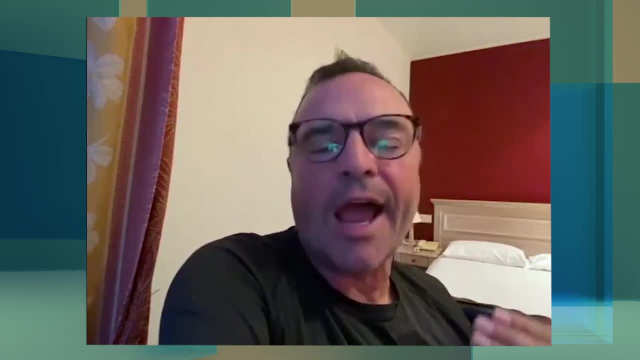 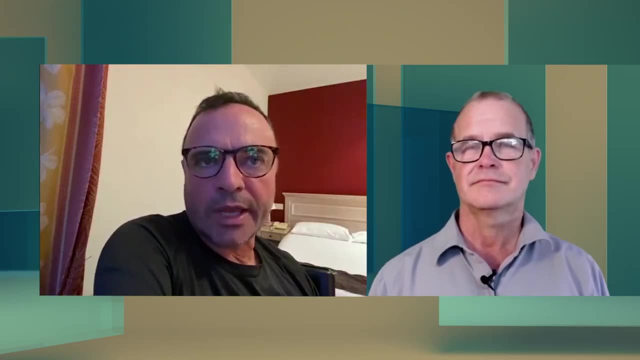 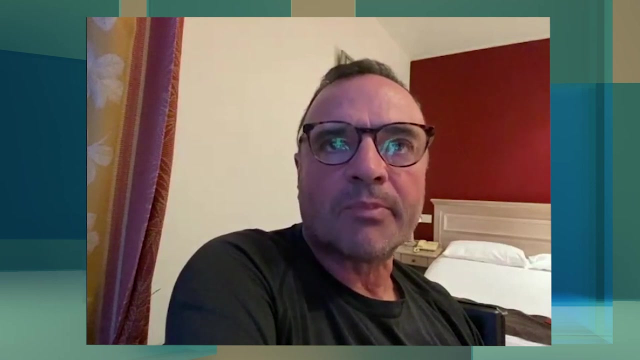 i'm always, uh, just doing a liter and a half. that's what works for me, a liter and a half of water, uh, and i set out. i'm very careful about what's in my pack. i usually carry an ipad with me but, um, the last couple times i had it with me, i just felt my pack was too heavy. 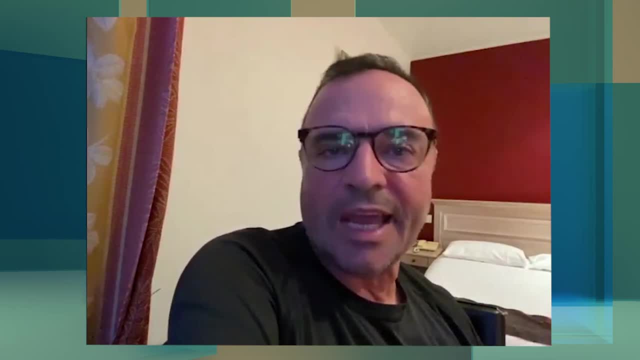 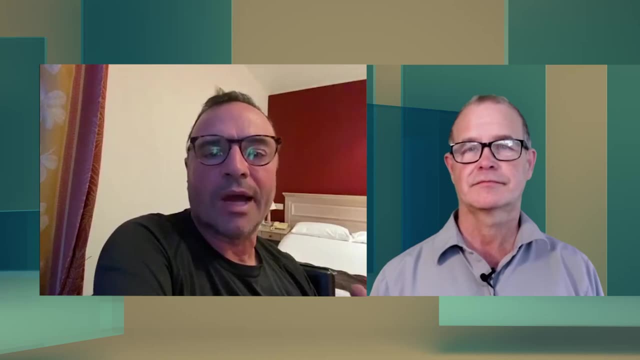 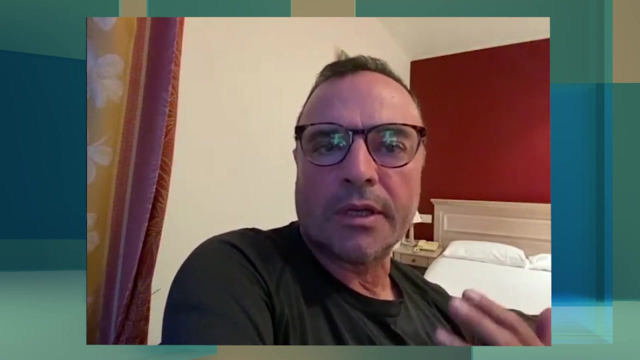 so i don't have my ipad with me, just a big camera, which is my only luxury really, but i need that for great photographs that will go into the guidebook. so i get my water and my food, and then i already have loaded the gps tracks onto my phone. 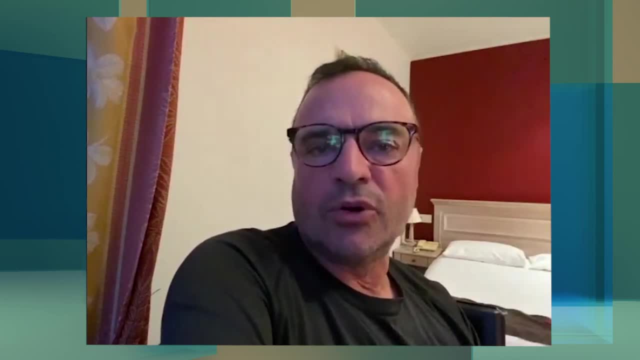 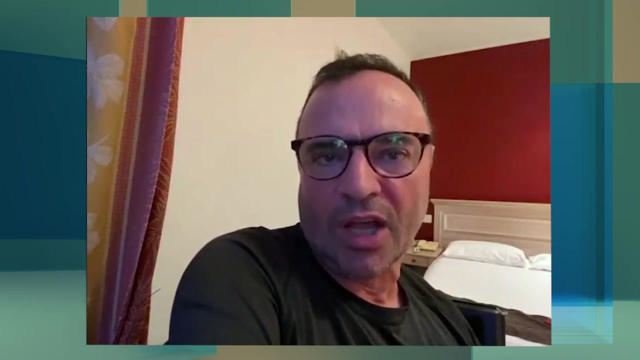 so i i open my phone when i step out the door and i turn on my gps and i follow the line through the day. or if i feel like, um, the line isn't making sense to me, then i make my own line. so, as an example here: 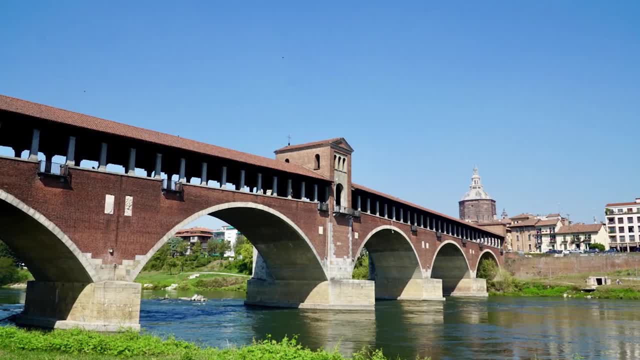 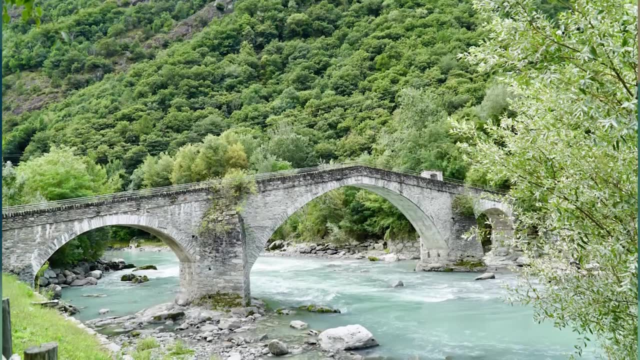 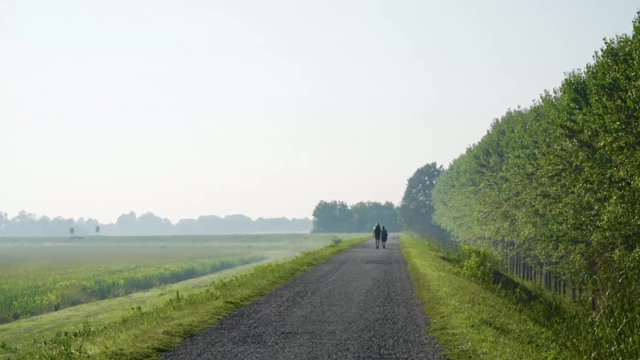 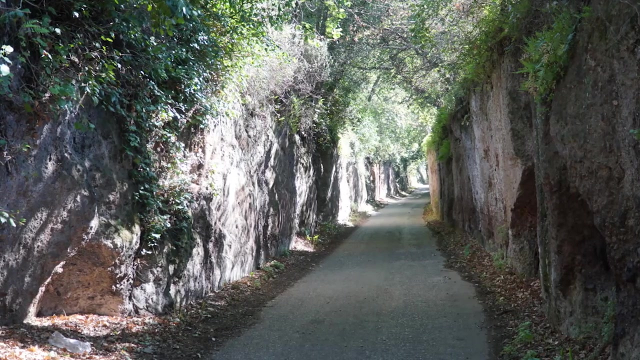 in france there are all these canals, and the canals usually have roads on either side and the very straight. well, their friend schuetzner sometimes runs out and goes into the woods and climbs a mountain and then comes back to the next city. well, if the canal connects the two cities, then, and it saves me five kilometers. 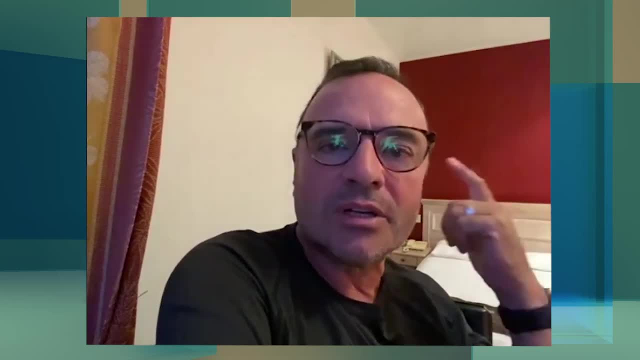 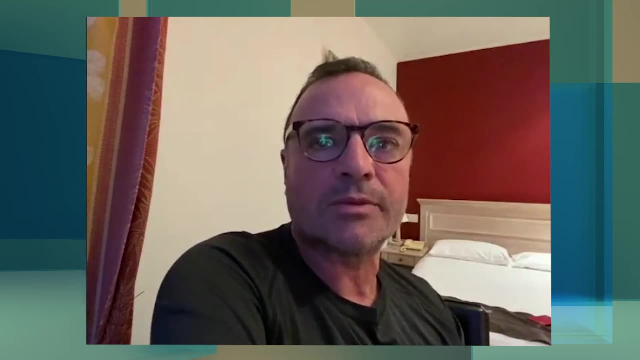 i'll probably take the canal road, so i'm um not just blindly following the route on my gps, but i'm also looking for the best options. i'm looking for photographs all the time because i'm looking for the best option for what i can take to the canal. 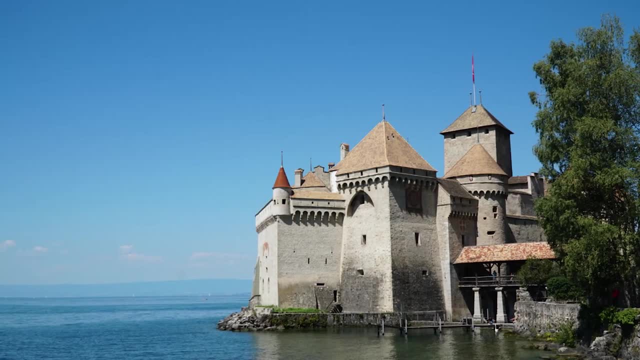 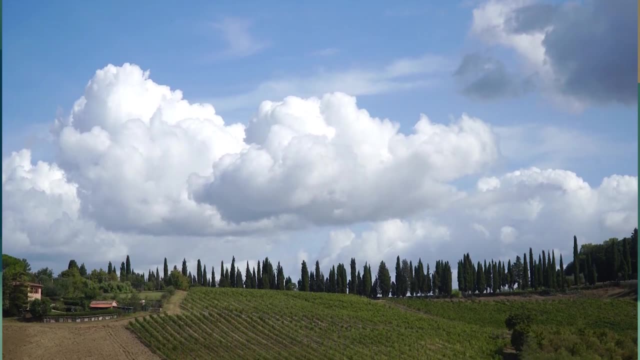 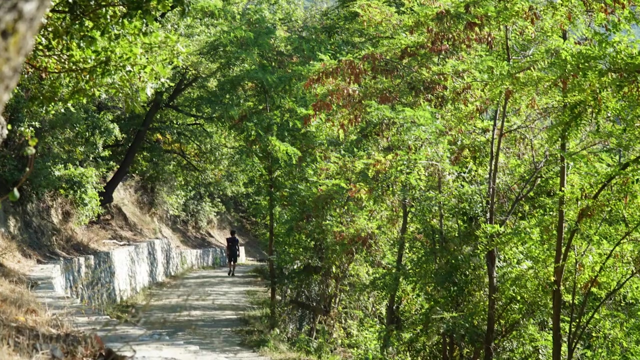 Because I think what makes a book great, other than the descriptions and the information, is photographs that are really compelling. Every town I go to, I'm looking for the great photograph And that's a part of guidebook writing that is underappreciated. 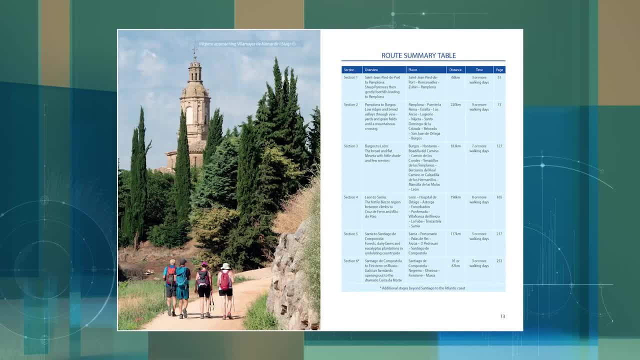 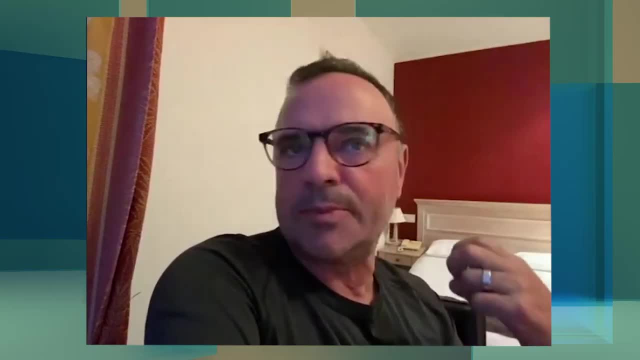 And when you see good photographs in a guidebook, then that's a very good thing. I really respect that. So a guidebook writer needs to be able to write, needs to be able to handle lots of data, needs to be able to handle things like a GPS and so on. 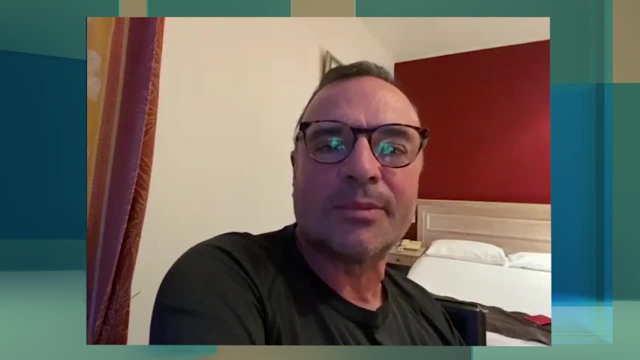 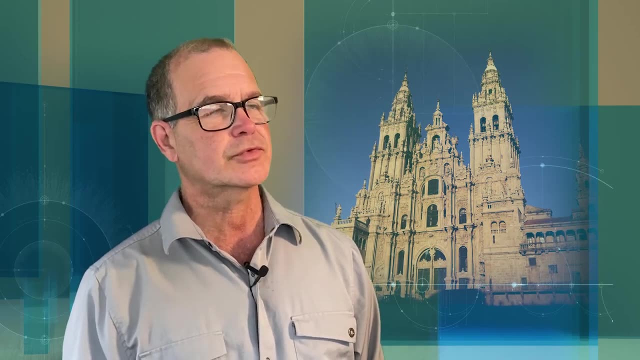 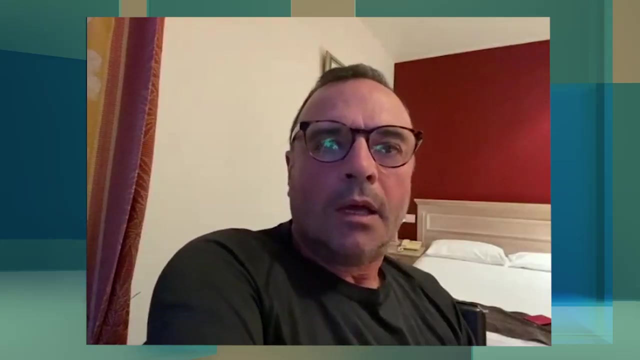 And then should have an artistic bent that allows them to do really high-quality photographs. Excellent, And so on different routes. would you book your accommodations ahead of time, And what sort of accommodations do you look for? Well, it all depends on the route. Okay Now, The last time I did the Camino Francis, I did not book my accommodations ahead until I got to Osobrero, And at Osobrero I couldn't find a good place. I ended up with my wife- which was great- in the municipal albergue at Osobrero, which probably has 150 beds. 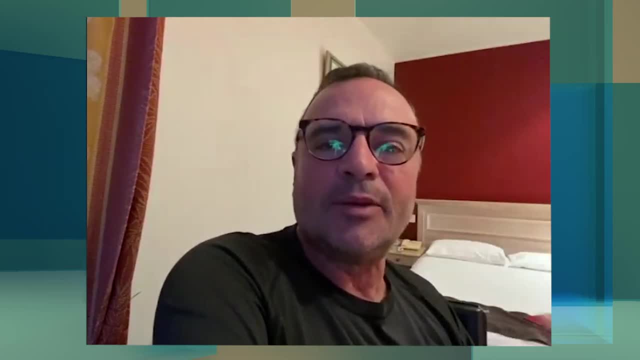 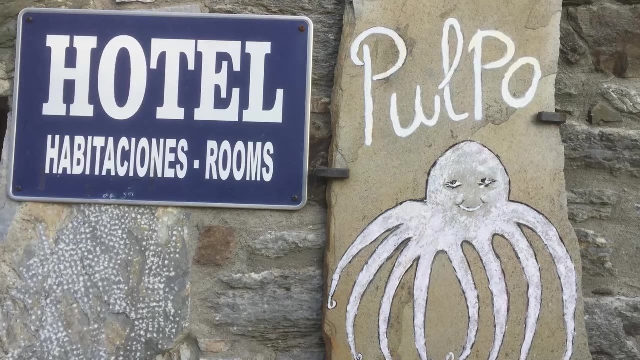 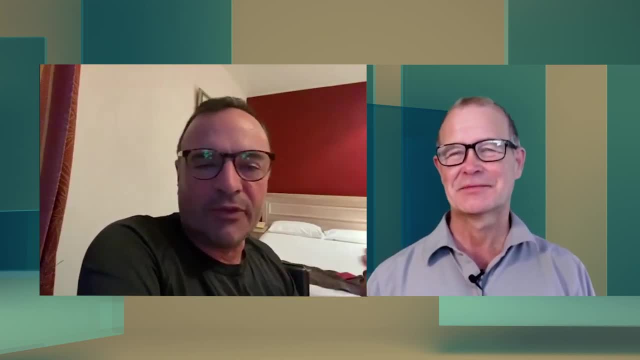 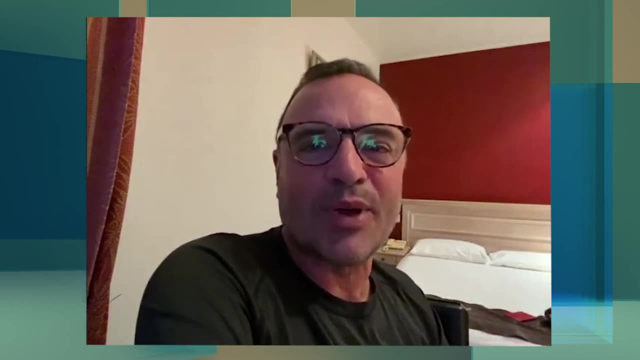 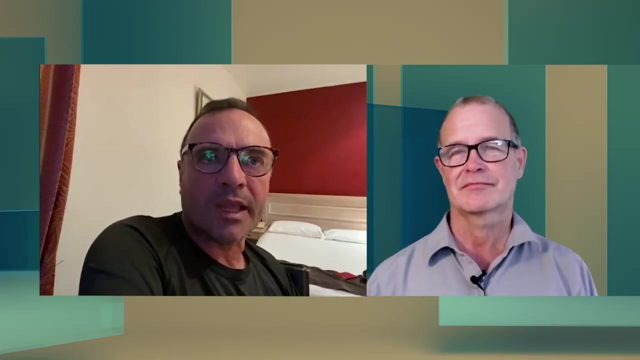 I want to go to the laundromat If I want to, I want to soak in the tub And I want good Wi-Fi. I want some privacy. I want some privacy also. So that's really my pattern: A hostel when I can find one and a hotel in the larger cities. 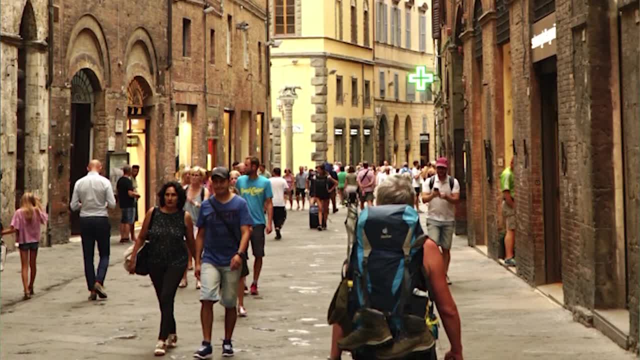 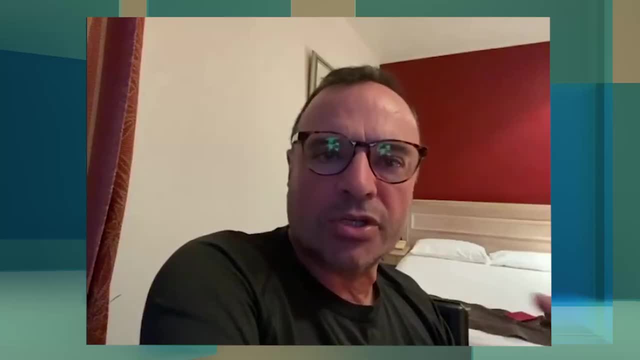 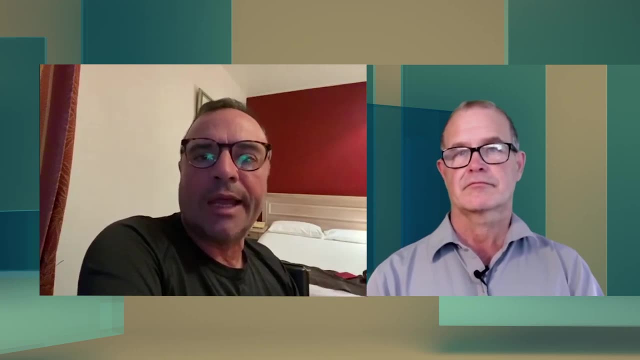 I usually book no more than about three or four nights ahead. So I have a day off tomorrow and I'm going to be planning my next week And the accommodations are kind of a challenge on the Via Francigena in France. So I will plan ahead my accommodations for five or six days. 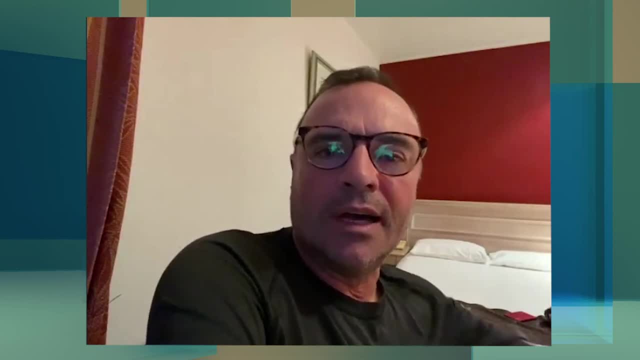 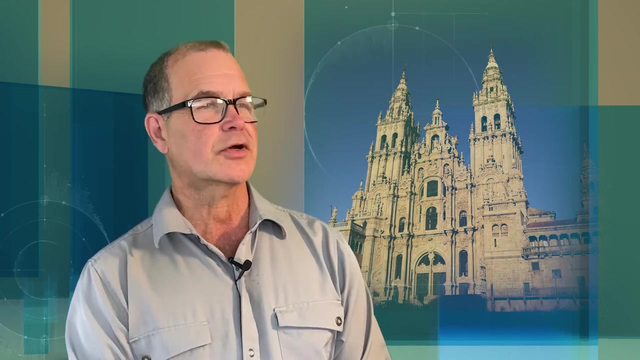 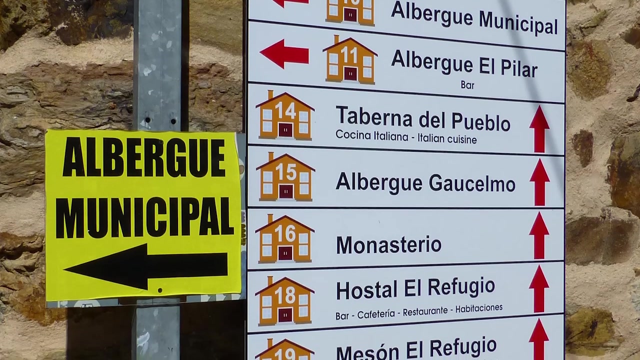 And then every night I'll look ahead to the fifth or sixth day beyond. I don't like to book accommodations, much more than that, because I want to retain my flexibility. So would that be the same on all routes? On the Francais, you can be more serendipitous, really, and just walk as long as you want to. 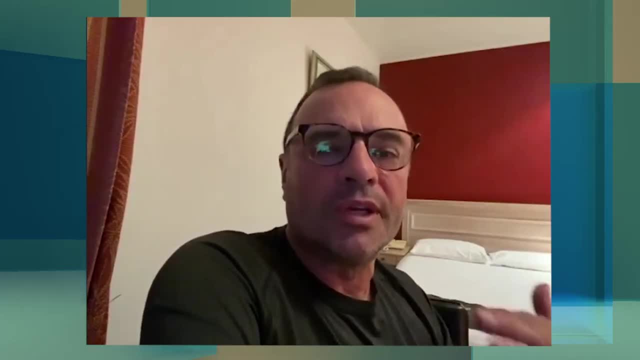 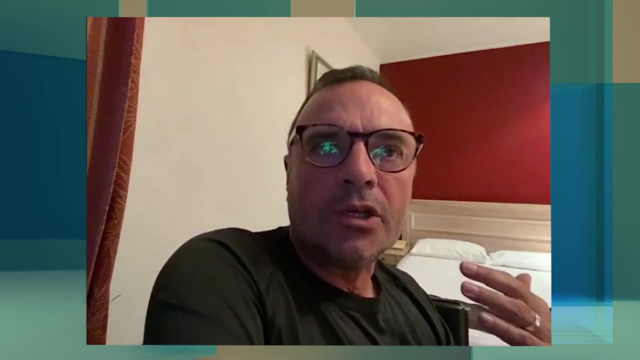 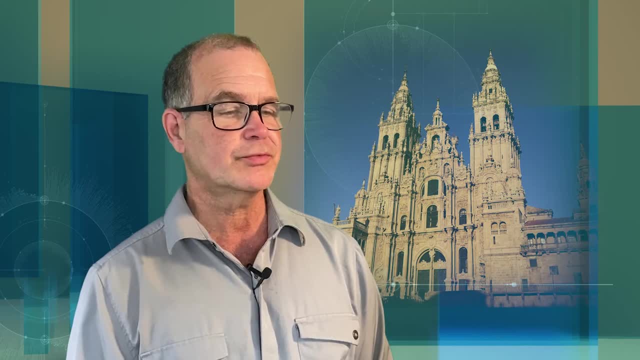 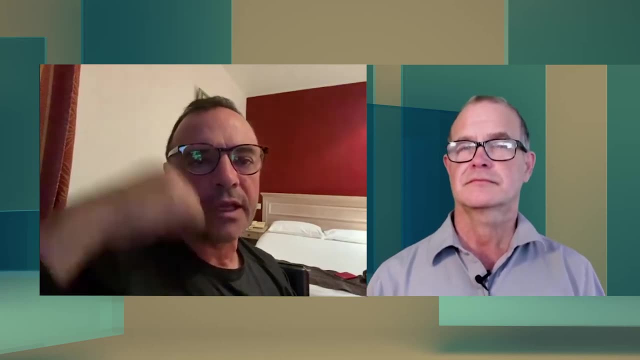 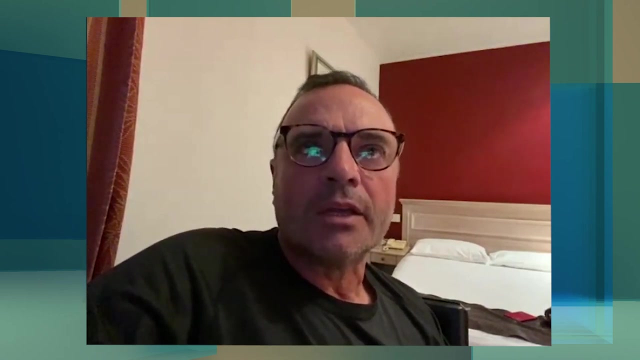 Let's talk about budget. How much money do people need and how much money do you spend? It's really different on the various different caminos. So on the Francais, I have a lot of money. I feel it's pretty easy to get by with about 40 to 50 euros a day. 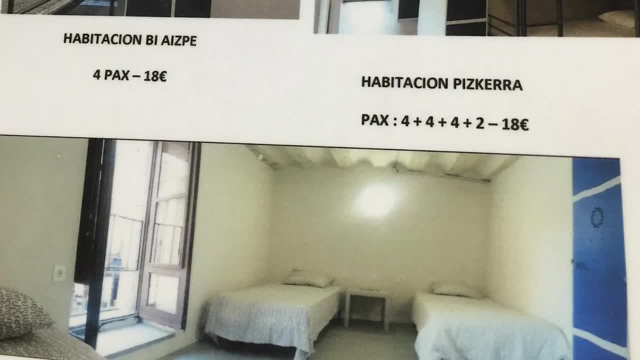 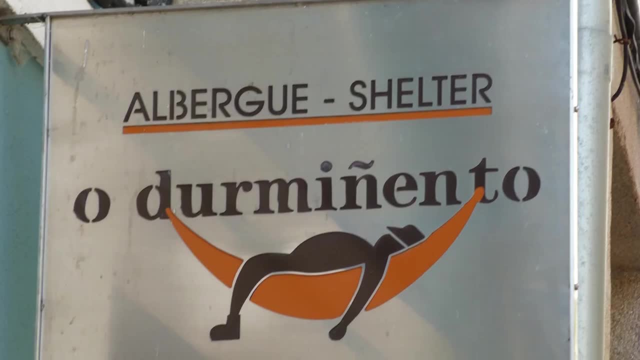 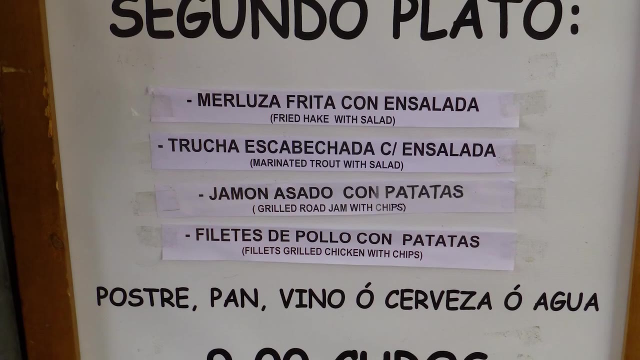 You can find accommodation usually for in the range of about 20 euros or less, depending on how picky you are about what the room is like- If you're in a large dormitory in a municipal- And then there are meals available for, say, 10 to 12 euros for a municipal. 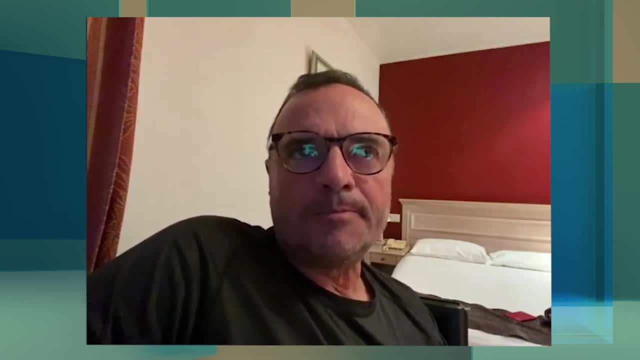 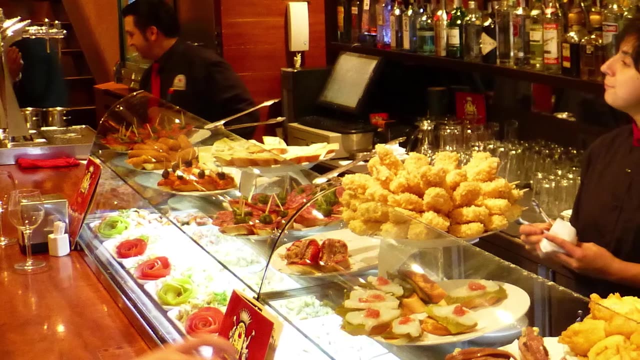 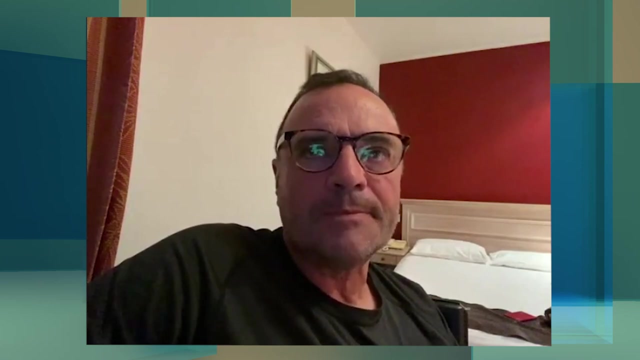 Then you get a new del Perugino, And so then it's lunch and breakfast besides that. So 40 to 50 euros is really doable. in the Francais, On the Franciscan, it's really different. So in France it's nice to be able to stay in a Gîte. 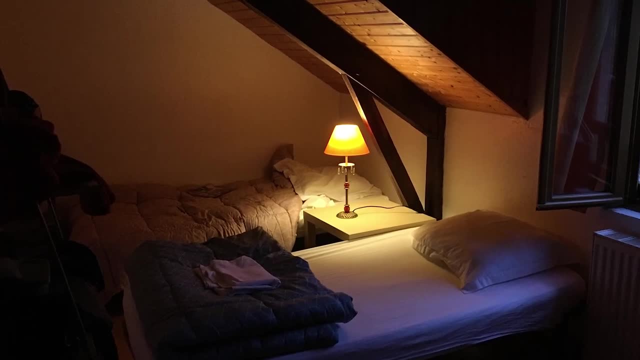 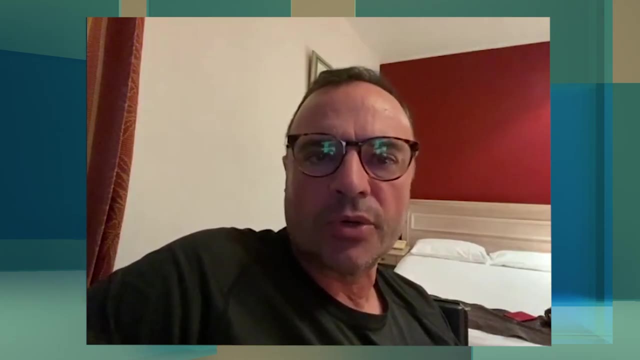 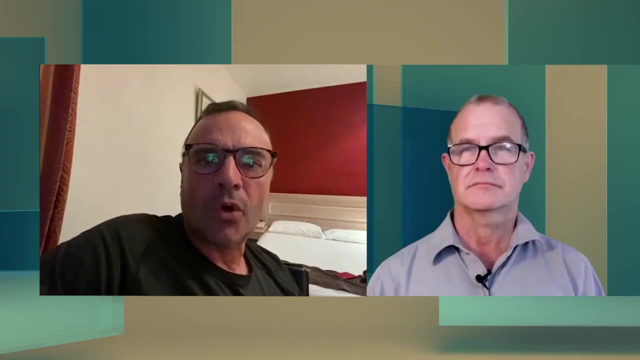 And a Gîte is oftentimes somebody's home or they've opened up a few bedrooms or it's sort of like a bed and breakfast. in some cases There are dormitory rooms, but oftentimes the host will offer demi-pension or half board. And then it's not uncommon with your overnight, your breakfast and your dinner to be in the range of about 60 to 70 euros a night. So on the Franciscan, that's probably a good amount to plan. There's also more camping available on the Franciscan. 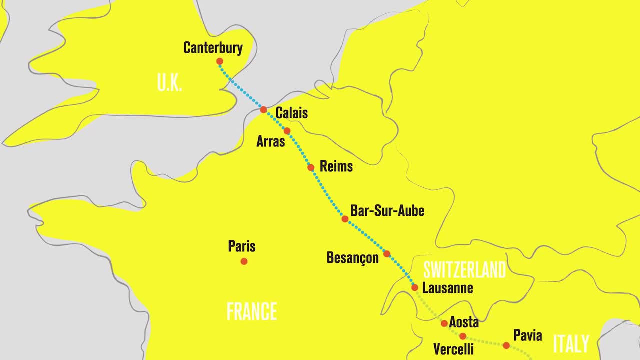 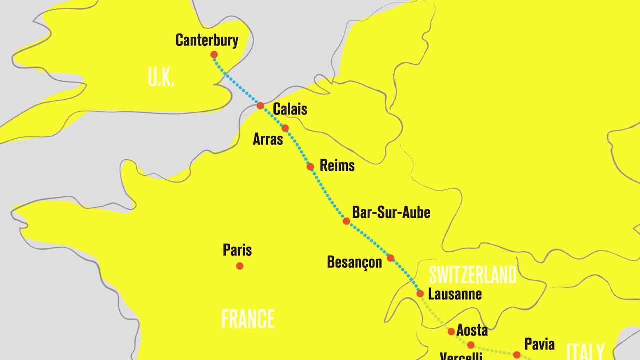 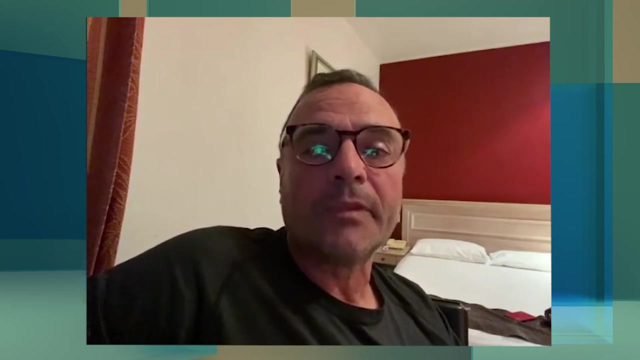 So oftentimes in France people will bring their tent, especially if they want to save some money on the long days. Basically it's 1,100 kilometers in France, So that's between 30 and 40 days And at 70 euros a night that's a lot of money. 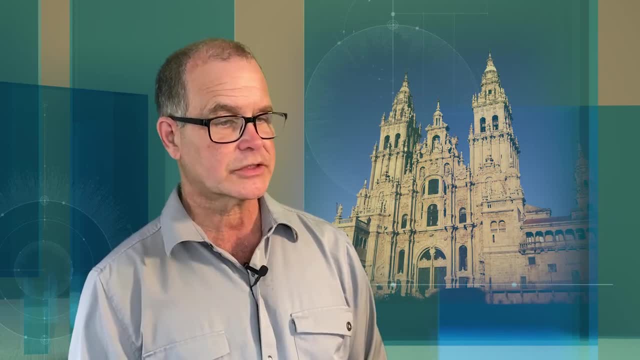 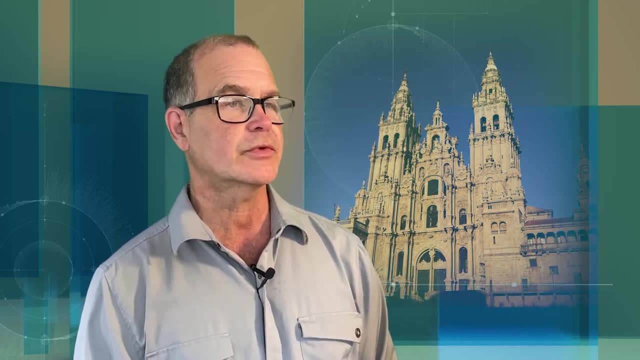 Yeah, We have a budget, usually because two of us are walking. We have a budget of about 40 to 60 euros a day And we find that Each or together Together, But we do that because we cook our own meals. 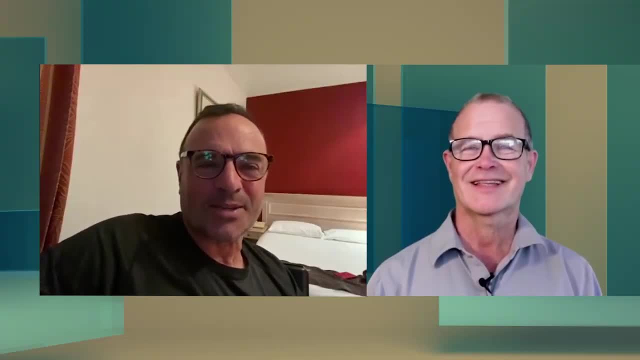 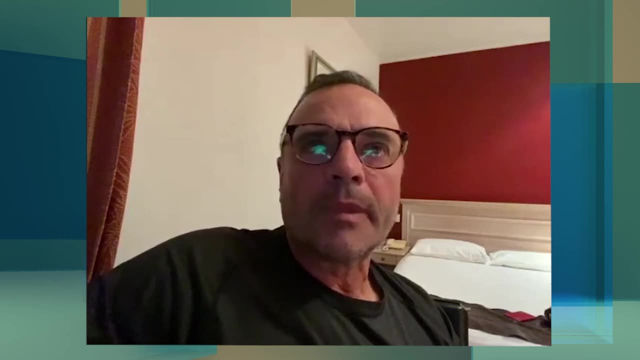 You're way more of a pilgrim than me, because by the end of the day- and I usually do 30 to 35 kilometer days- It's not uncommon for me, But I want somebody to bring my dinner to me, Okay. 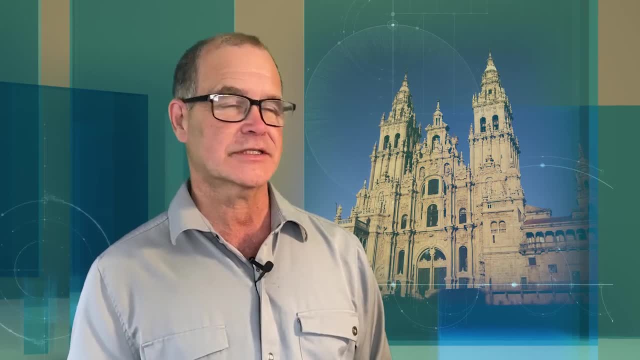 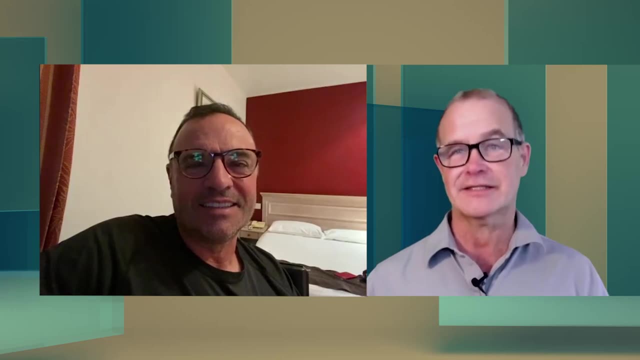 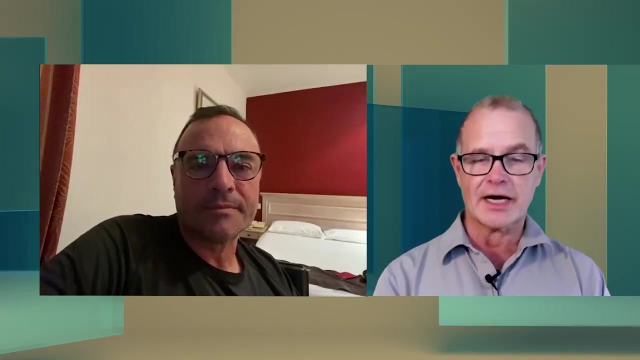 And in France because the food is exceptional. especially the food is so exceptional sometimes it's worth it to have a very fancy pilgrimage versus budget conscious pilgrimage. So can you tell us some highlights about some of the walks that you've done? And that's a very open question. 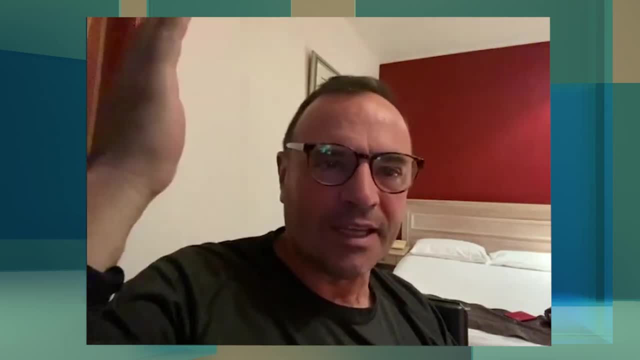 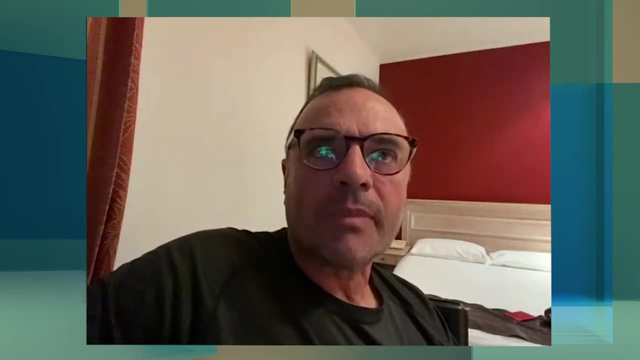 Sure is, But immediately Some come to mind, and oftentimes they're in the mountains. So one of the reasons that I'd like to be a Franciscan or so much, is crossing the great St Bernard pass. So, St Bernard, everybody knows dogs. 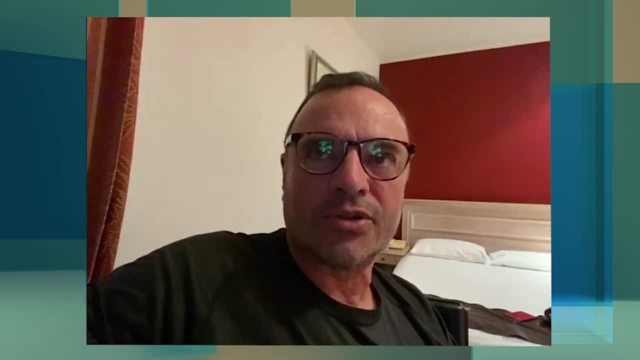 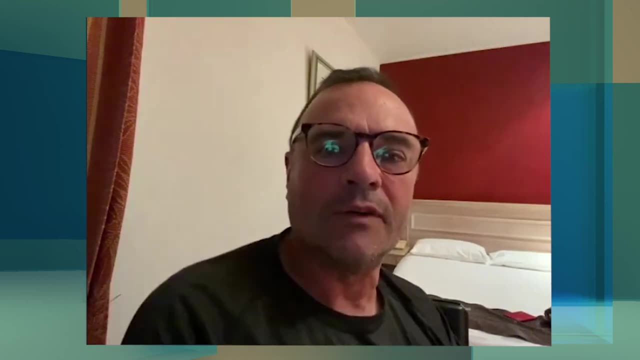 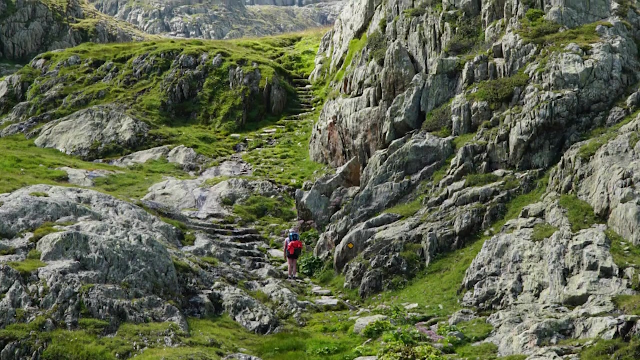 Well, sure enough, the dogs were bred in order to help travelers over the mountain pass that now bears the name of the saints- Okay, St Bernard, who, a thousand years ago, established a hospice at the top, And then, hundreds of years later, they started using St. 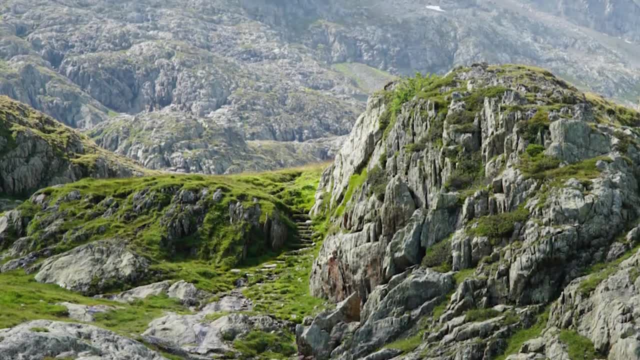 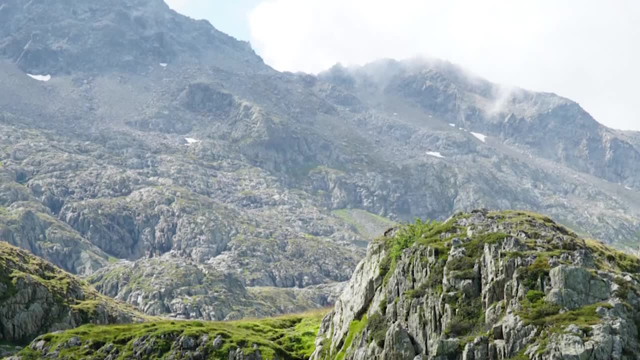 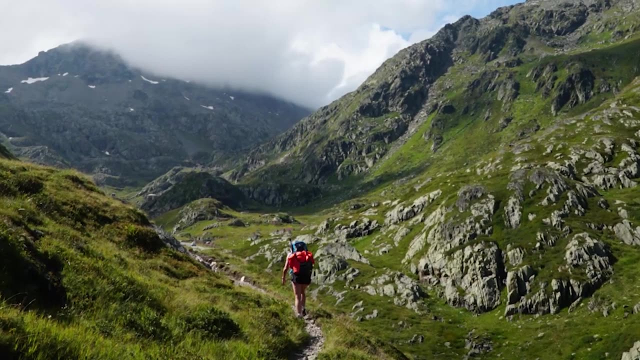 Bernard dogs for rescue. But I'll tell you, the three or four days leading up to summiting, the great St Bernard pass, which is 2400 meters, about 8,400 feet, is pristine, beautiful And it's just an amazing view. 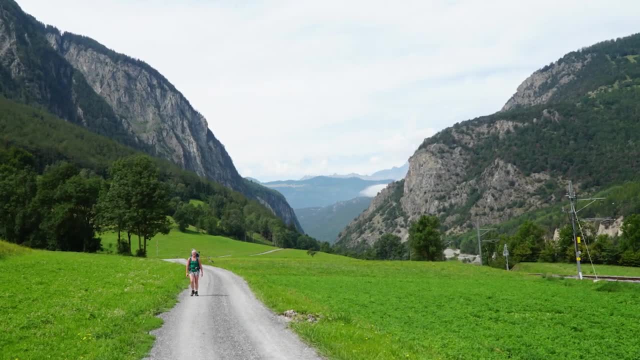 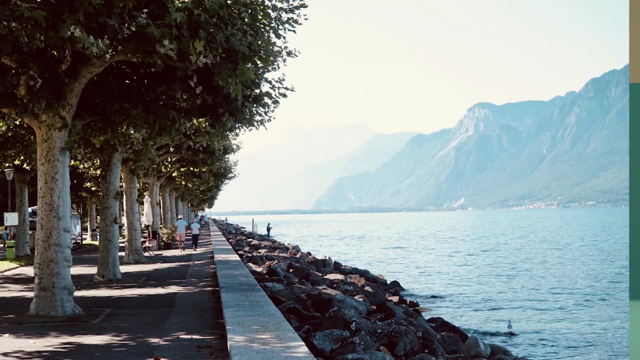 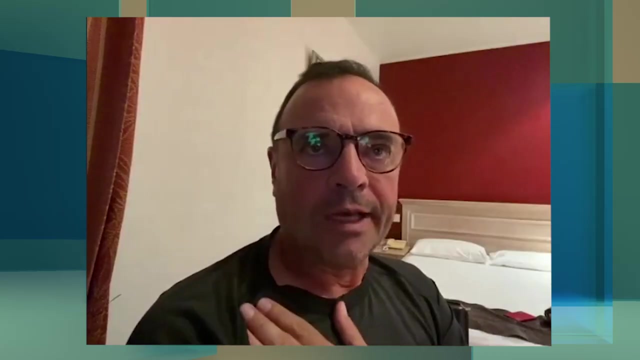 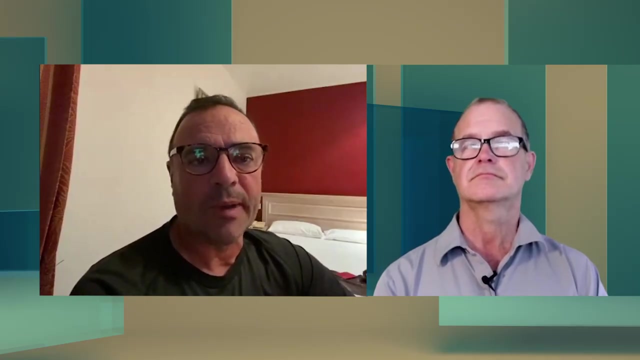 But I know that they're walking. And then you get to the pass and here are jagged granite peaks and the lake. You're standing in Switzerland, You can see a hundred yards away to Italy And it's just spectacular. Then the next day down- actually, the next four or five days- are also through the mountains. 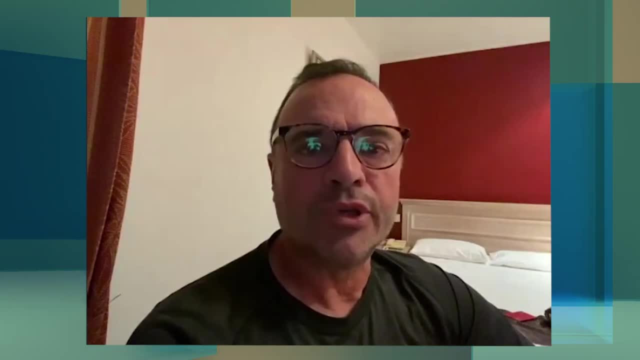 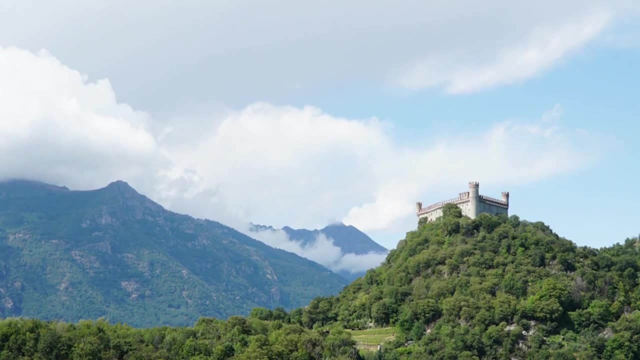 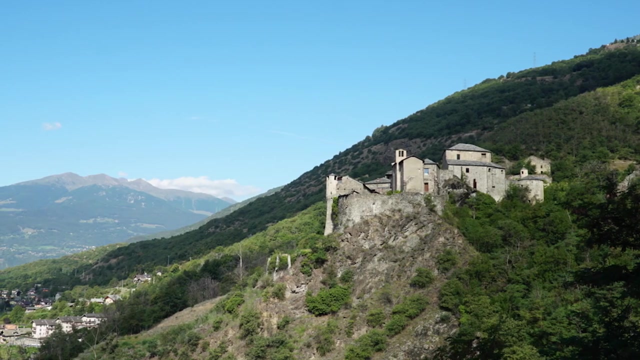 And oftentimes there are just beautiful uh forests and mountains, and italy has all kinds of castles. you can probably go by eight or ten castles over the next uh seven or eight days. so those are two of the really outstanding and wonderful things i see on the francis. 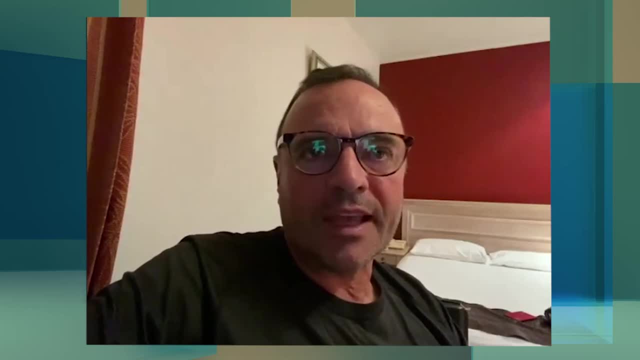 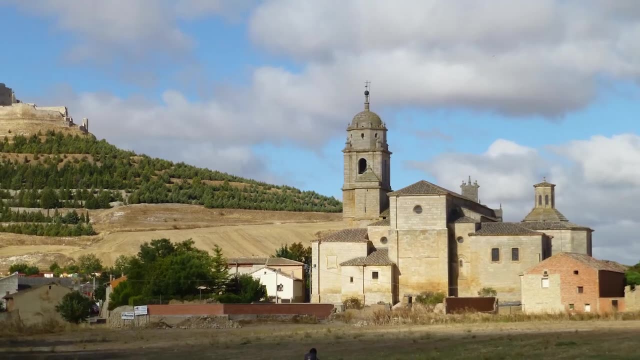 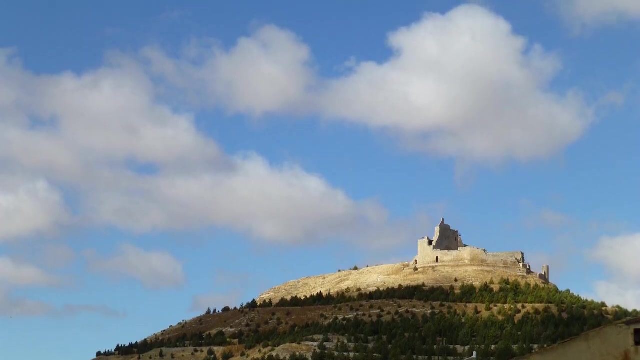 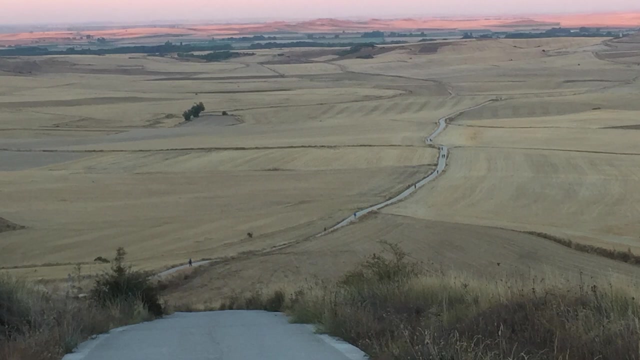 on the francis, i think, uh, you know the meseta doesn't get good enough, uh, reviews. but when i talk about that moment with nature, an example of that is after castro jerez, when you go up to the height, uh, where you look down on the valley toward ituro de la vega, you can see i'm 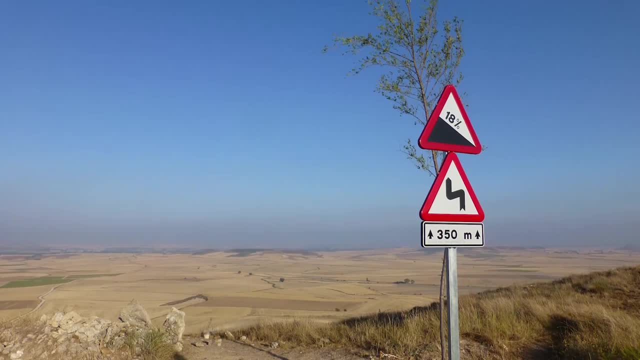 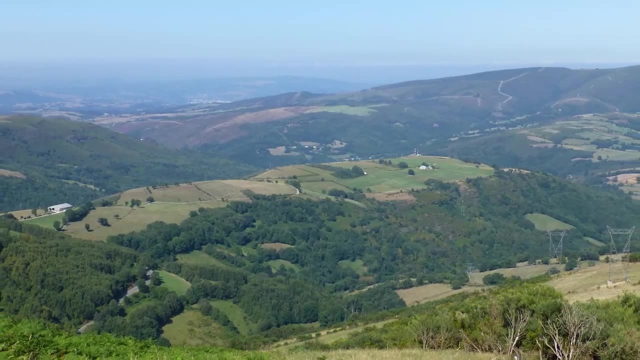 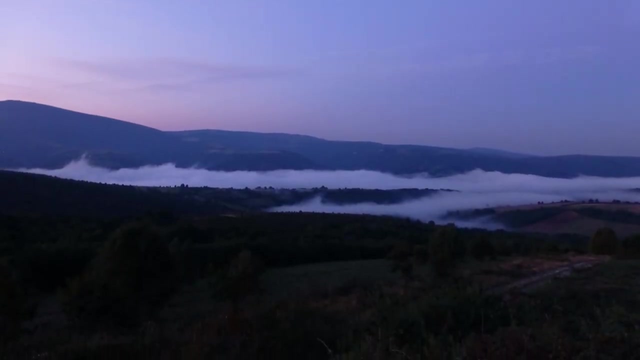 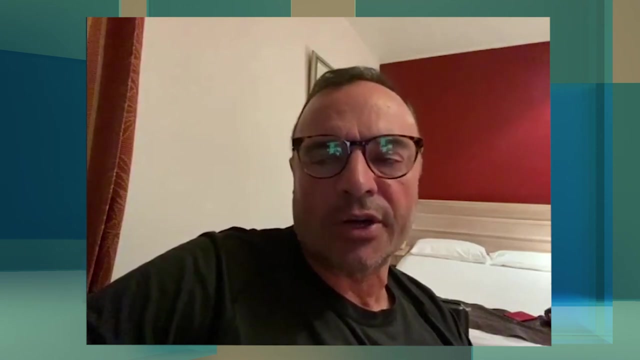 sure, 10 to 15 miles and it's a patchwork of farms. it's really spectacular. you also get that experience at osoboro. after uh, you're starting your way down toward tria castella and it's just beautiful to be in the mountain areas like that. everybody loves finisterre, everybody. 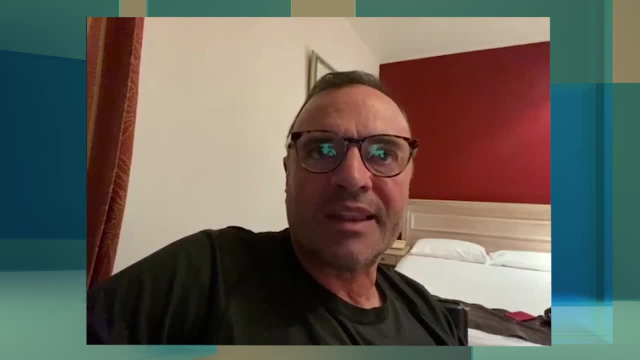 loves muxia. but what about the quiet beaches between finisterre and muxia? i encourage people, take that walk, there's a lot to see. and take some extra time so you can walk the 20 minutes or so to one of the great exclusive i guess you could say. uh, small beaches where nobody else goes. you're almost certain to be all by. 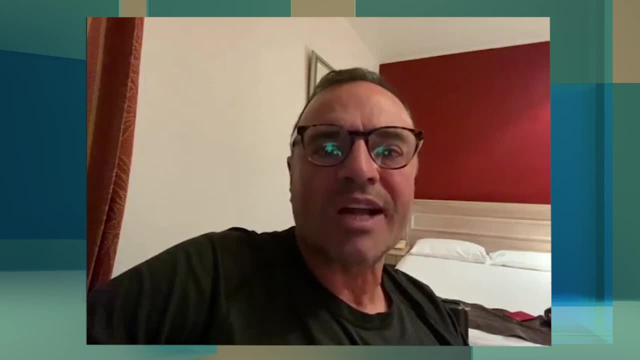 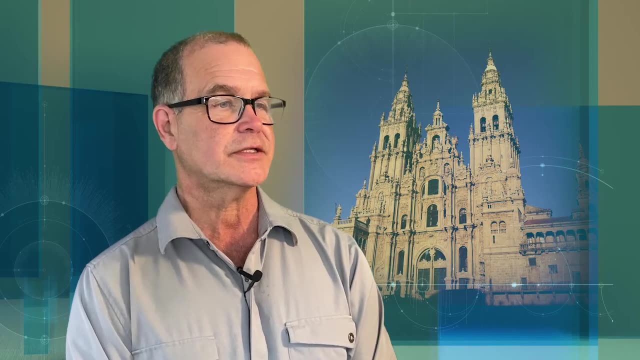 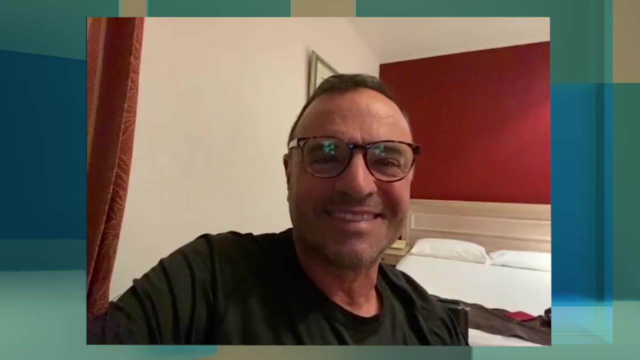 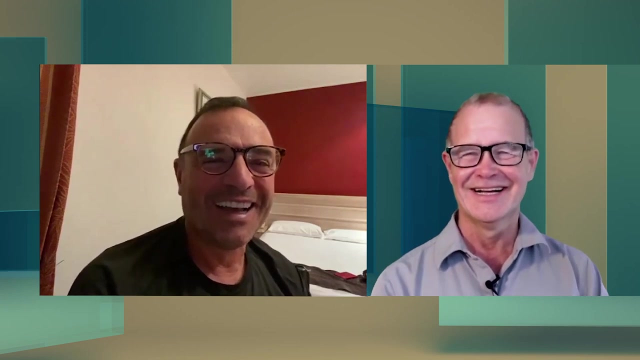 yourself and, uh, you can enjoy the crashing of the waves there. so those are some of the great places i've seen. so, uh, in the final question, uh, sandy, did you ever have any language difficulties while you were traveling? i have language difficulties every single day, but to me that's part of the fun. so, um, i'm also. 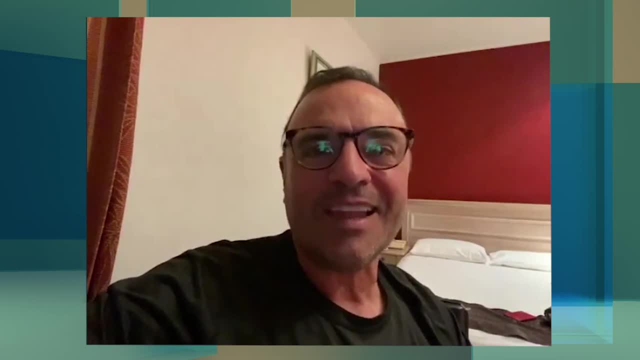 working on the guidebook in california, and it's really fun to see the difference between being in a place where you speak the language and being in a place where sometimes you don't have the language, you don't really know what's going on around you, and so, between french, spanish and 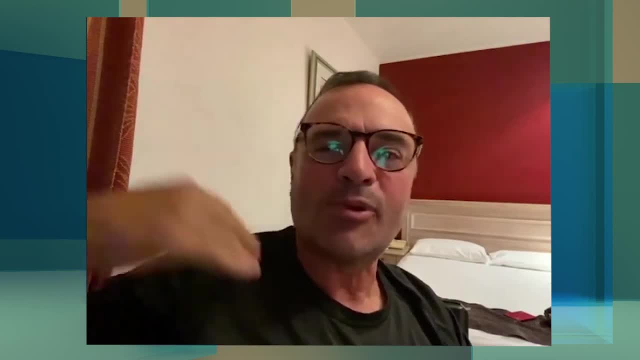 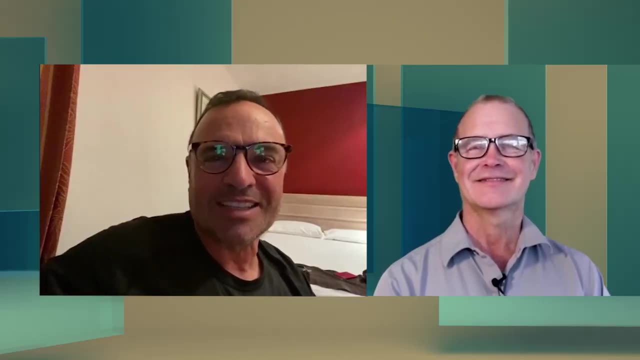 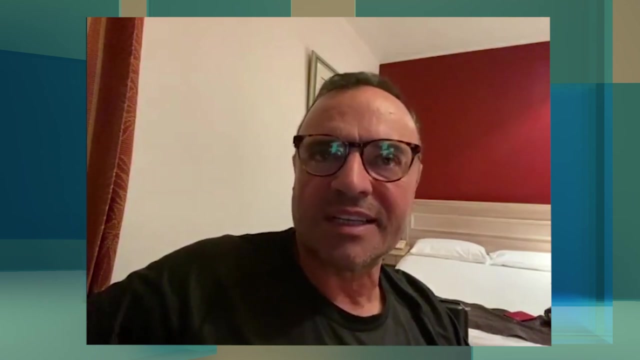 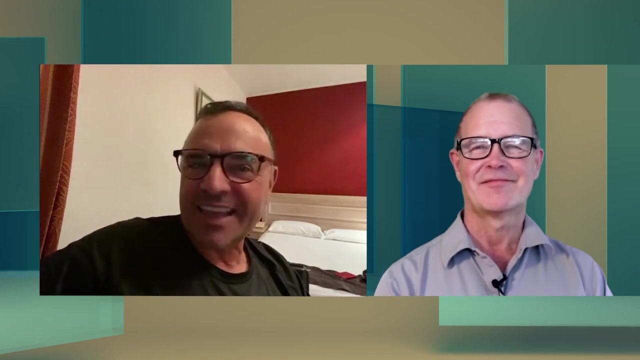 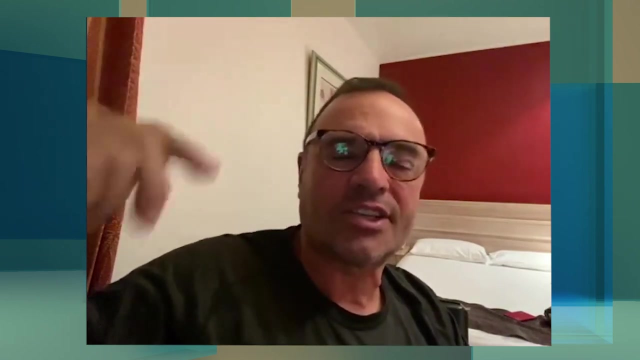 italian. i can usually, uh, come up with my own romance language words based on one of those three that make absolutely no sense to anybody. but the average pilgrim has something that i didn't have when i started in 2008, and that is google translate. uh, get the app. it's free, and you can even download the italian, spanish, french dictionaries. 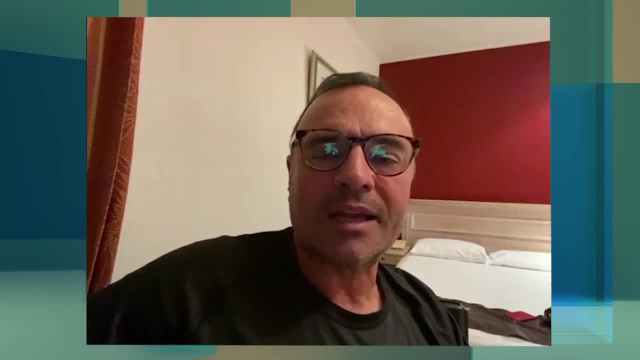 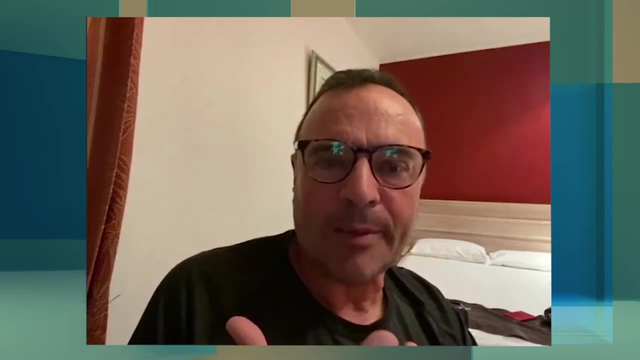 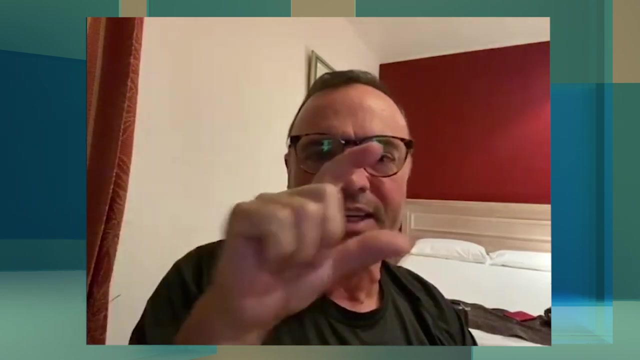 so you don't need a cell connection to make um translations for you and uh, then you can speak into it. you don't even need to type it. it will think for a minute and then it will give you the translation. when you turn it around, it's big enough for the person on the other side of the 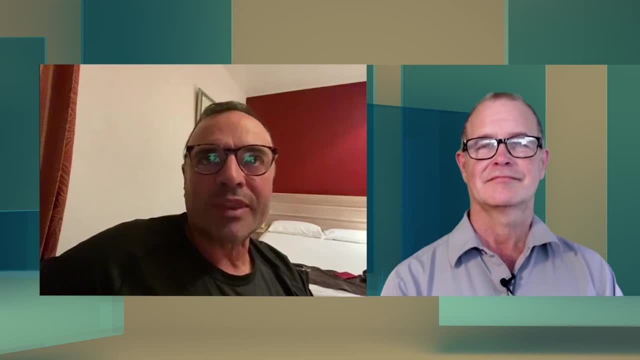 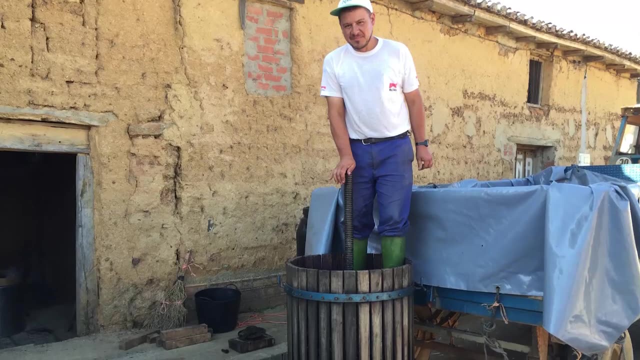 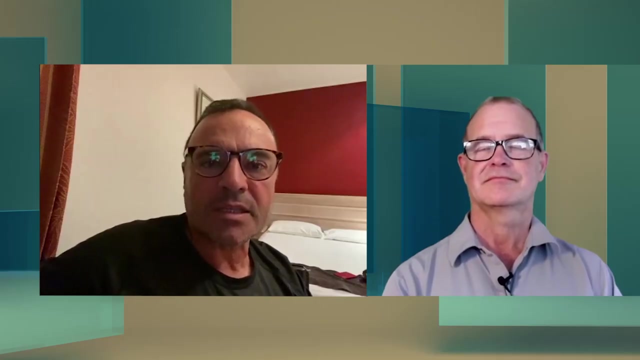 counter to be able to translate it, and you can even download the italian, spanish, french dictionaries to be able to read. so i don't think there's much excuse anymore for people not being able to be understood. but i i also believe it really is out of respect that still a person should learn. 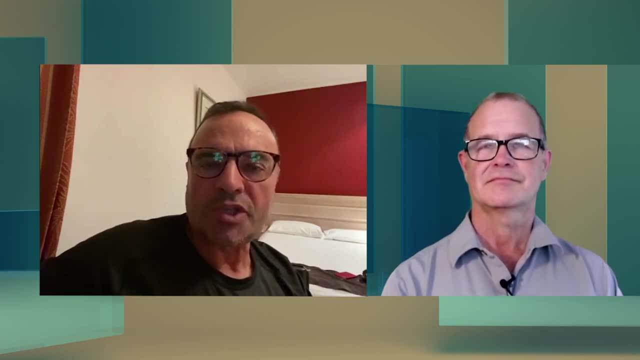 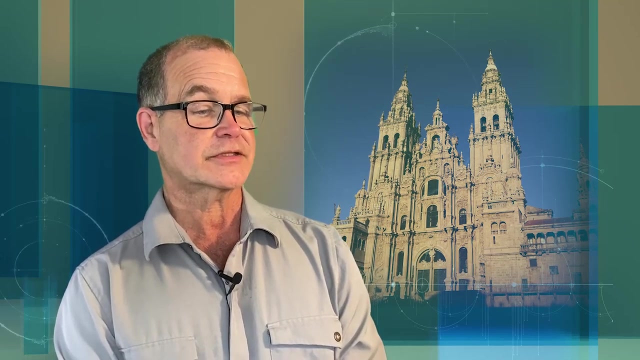 as much as they can of the language before they go, and that earns affection and respect. so i think it's still important for people to try to learn some and then use google translate when you get in trouble. so can you tell us a little bit about the best albergue that you've ever? 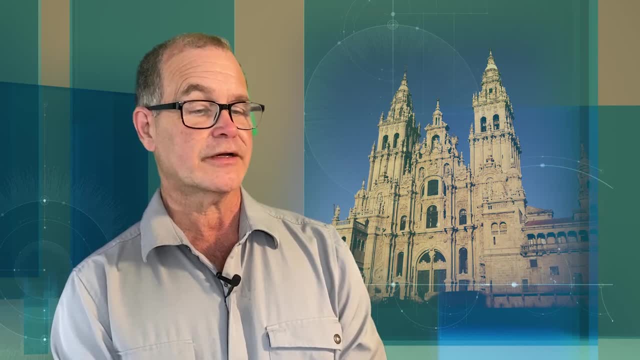 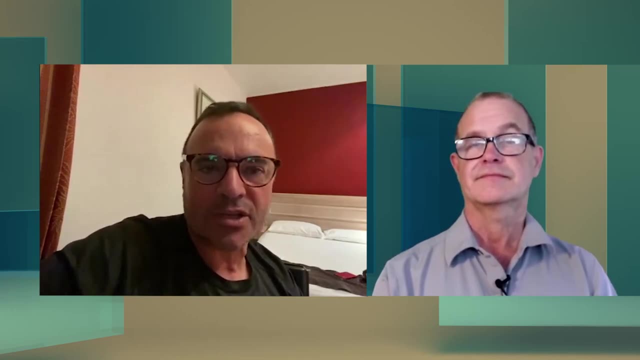 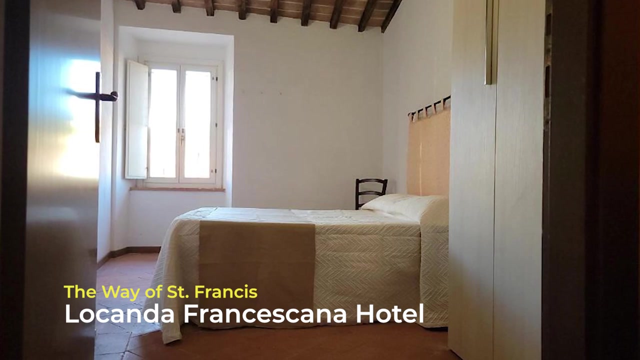 stayed in, and specifically one on the way of saint francis. well, on the way of saint francis, my favorite place to stay is a place called locanda francescana in poggio bastone. there is the owner. it's a private place. the owner's name is feliciano and he takes great 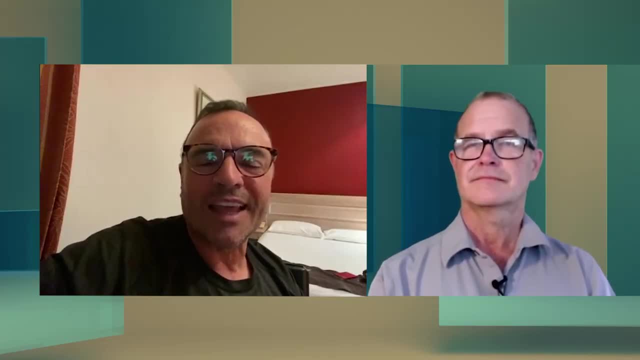 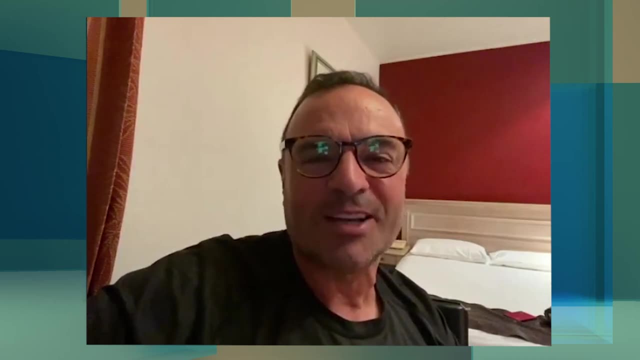 care of the pilgrims that come through. but what i like best is that at the restaurant where he serves the pilgrims his mother is the cook, so we get to meet his mother, have some real local italian food and have a fun, friendly visit with feliciano. excellent, is there another? uh? 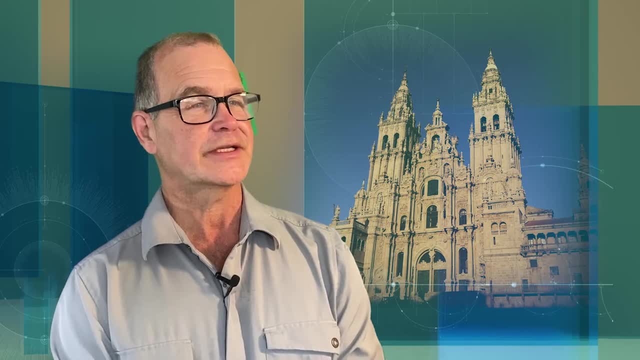 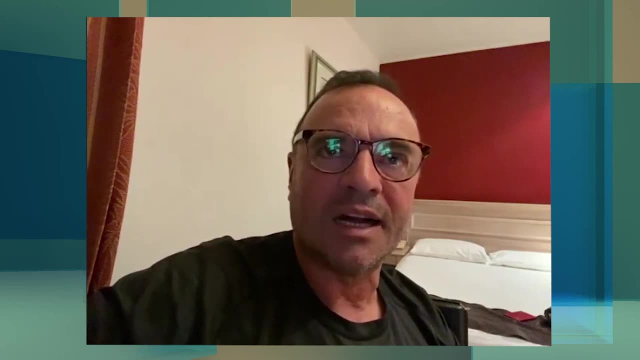 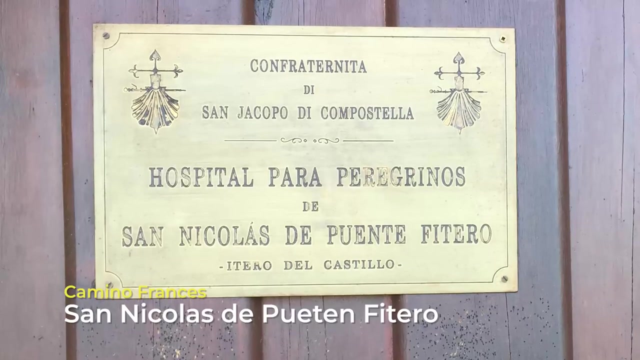 albergue that really comes to mind when you see the best albergue that you've been in. oh, my favorite albergue of any camino is the uh san nicola at puente fichero on the camino francis. now that's the albergue that's in the old pilgrim hospital. 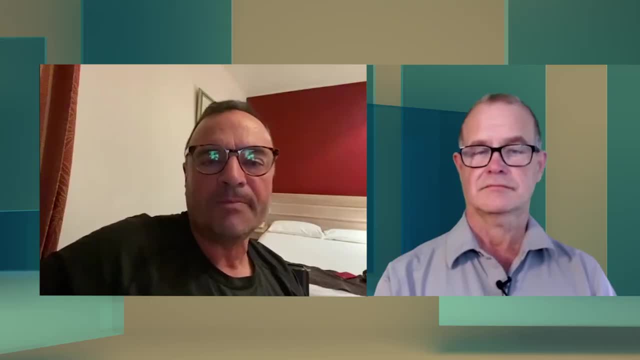 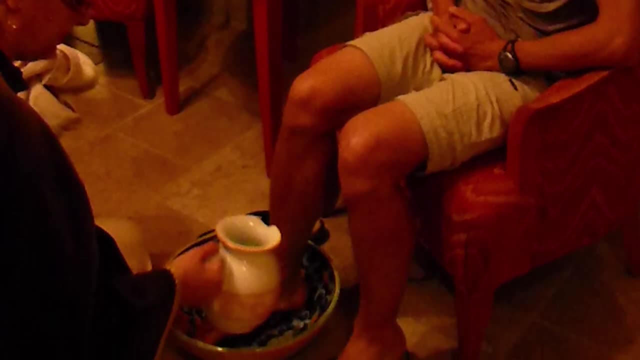 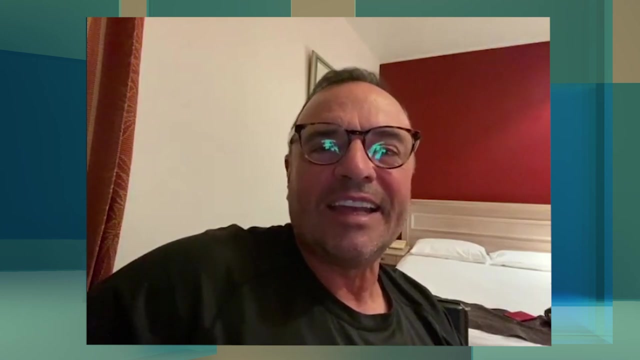 and it's run by the italian confraternity. they only have about 30 people a night that can stay there and they wash your feet and say a prayer and then cook you a spaghetti dinner and have a wine drinking competition. so between those things it just is the funnest atmosphere and the most, um, the most sort of intimate. 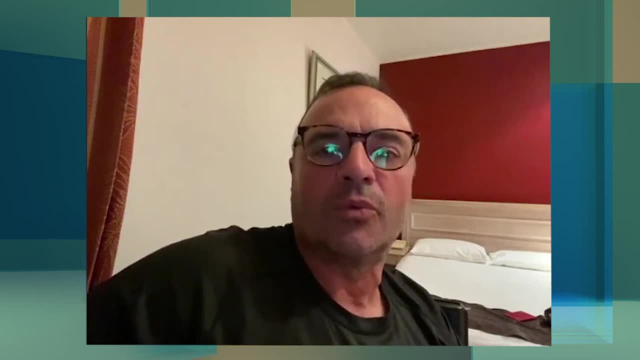 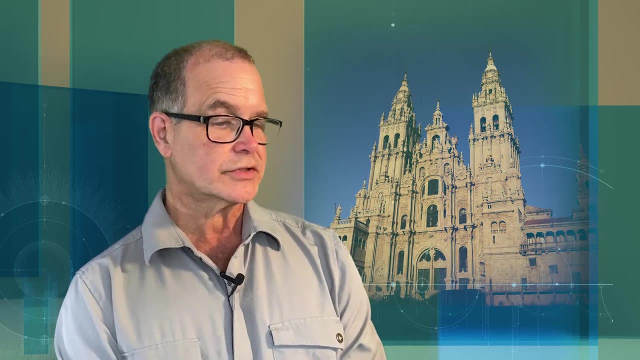 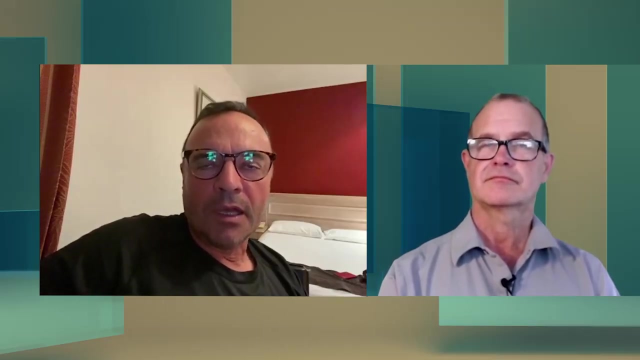 and loving place to be in, the communal meal, the foot washing and the fun that you have in that little remote location. okay, excellent. which route is mostly done on backcountry roads or trails? i would say that um of the routes that i have done, both the via francisana and the via de francisco- are mostly on backcountry roads and trails. 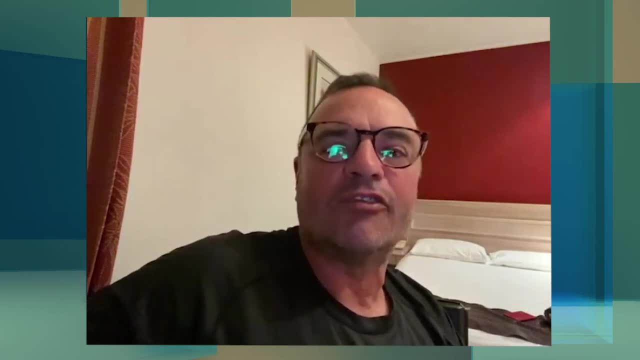 so france and italy seem to have more backcountry roads than places like the united states. um, in spain there also are. the funny thing about the camino francis is that the roads feel like they're pedestrian walkways. they stop feeling like country roads and they're really. 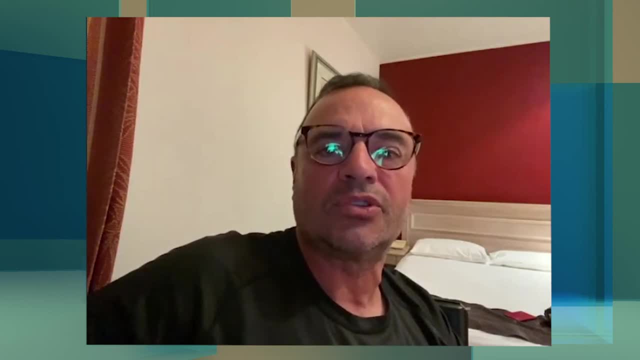 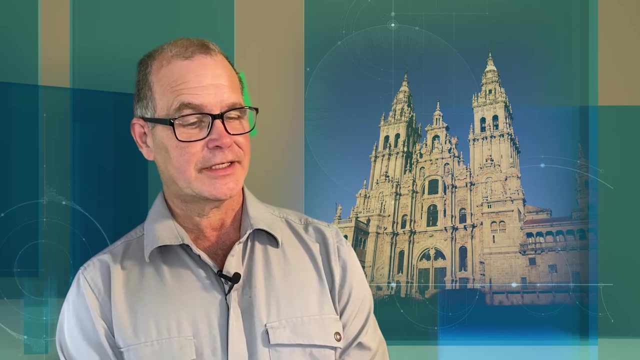 they're made for lots and lots of pilgrims to be able to cross. so i would have to say the francisana and the francesco are the ones that are most like that. uh, the next question is uh rather funny. if one can speak spanish, can you get heard in italy? 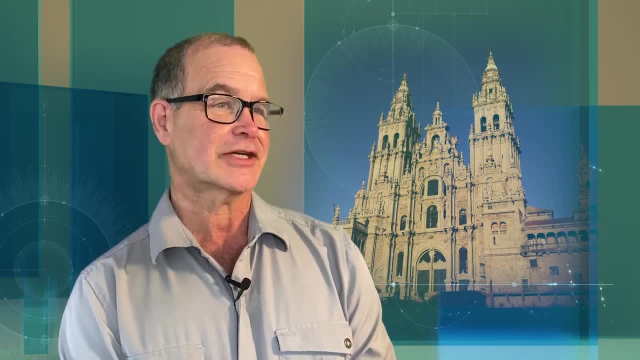 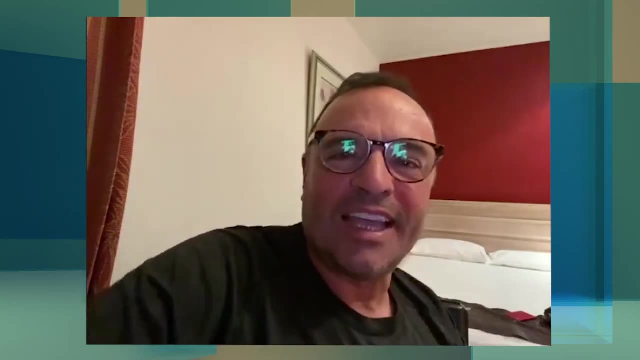 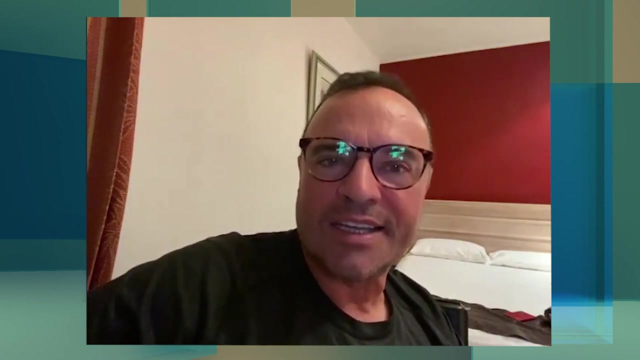 when you speak a little bit louder, with more hand gestures, or do you actually have to learn italian? that's great. you know the before i learned any italian at all, i used my spanish and i was surprised how much was understood when i took italian classes. there was a priest from argentina who came in in the third week. 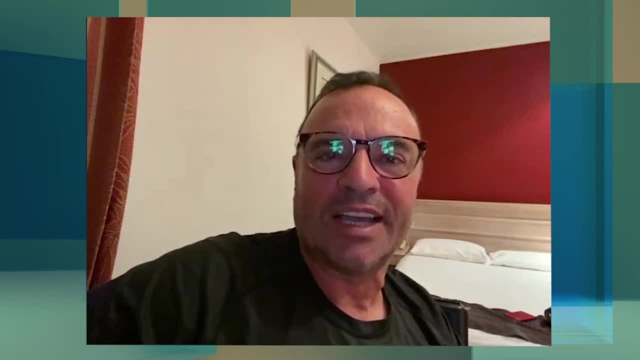 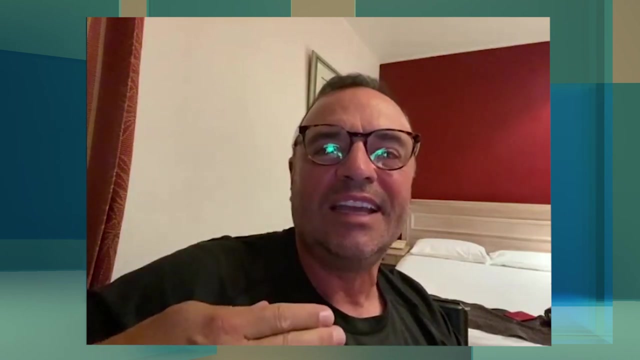 and by about the second day he was already better at italian than i was after two weeks. so you definitely have a leg up in italy. if you have strong spanish and if you're a native spanish speaker, you'll intrinsically be able to make sense of a lot of the things that you're talking about. 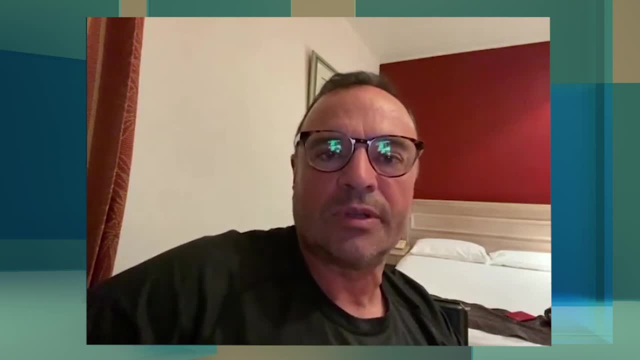 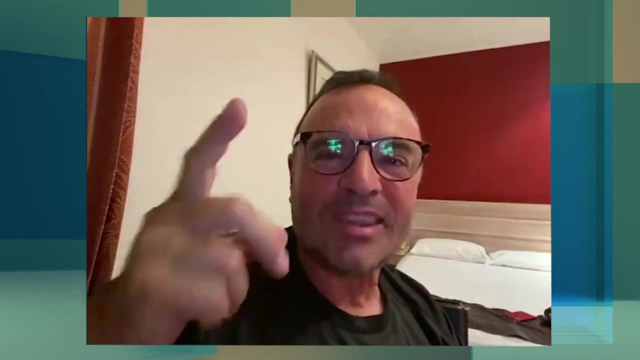 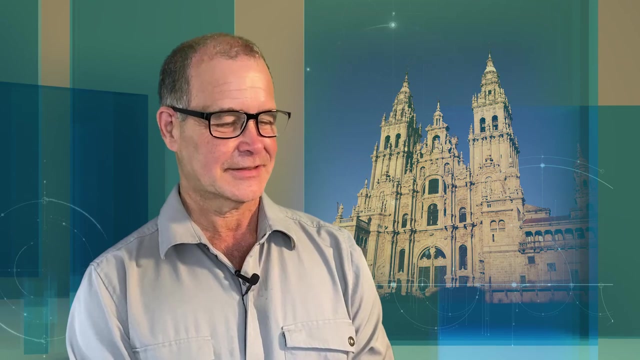 italian and the. the same is true the other way. so, as far as the loudness of voice, i'm not sure that's helpful, but i know that in italy the gestures are helpful, because that's how much their speaking happens too. yes, uh, i have an italian friend that i told them that if we ever 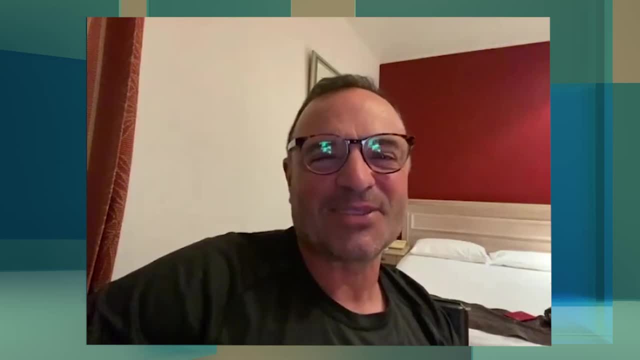 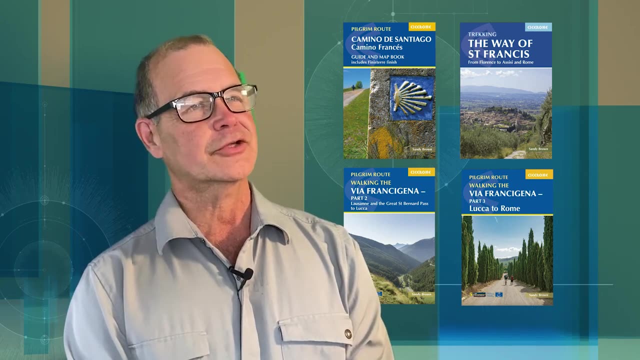 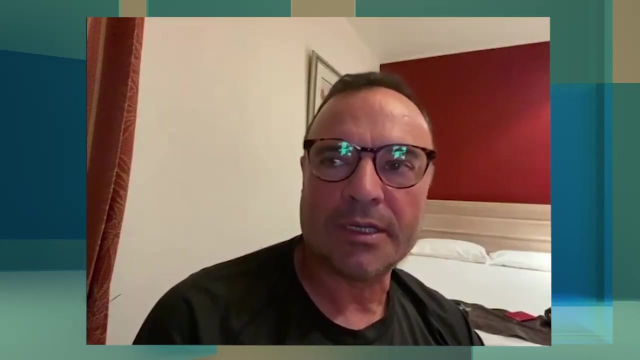 tied their hands together, they couldn't speak. that's right, exactly, exactly. so if people want to buy your guidebooks or see them, how would they get access to them? well, it's very easy to do on amazon, and i guess amazon in canada is amazonca, right? yes, okay, so you can. 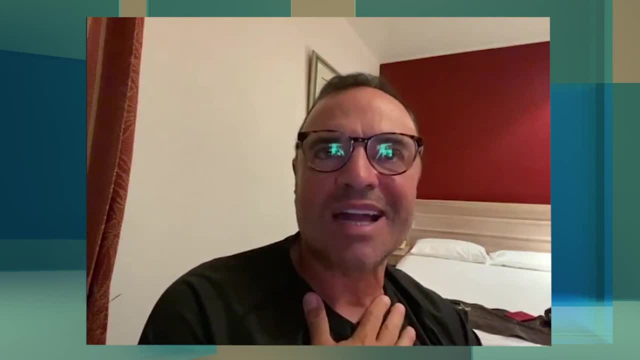 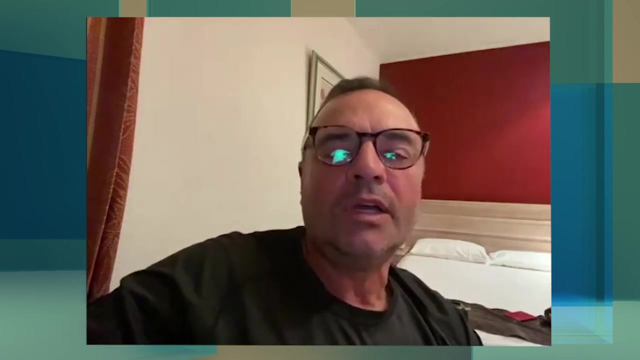 go and get them on amazon. as it turns out, amazon is not that good at making the most of the best content for the public, so the best way is to go to the website ciceronecouk. and that's the ciceronecouk website. and that's the ciceronecouk website. 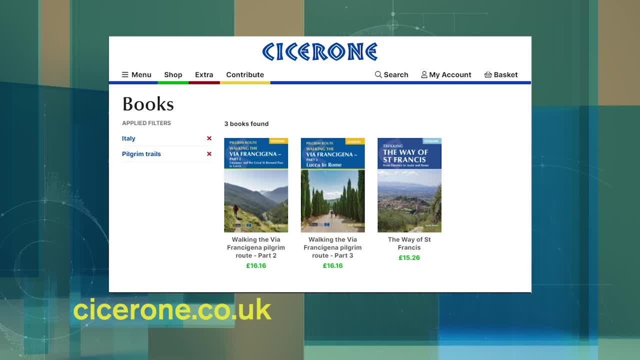 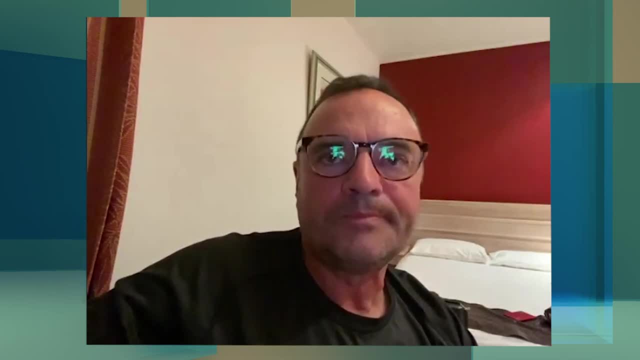 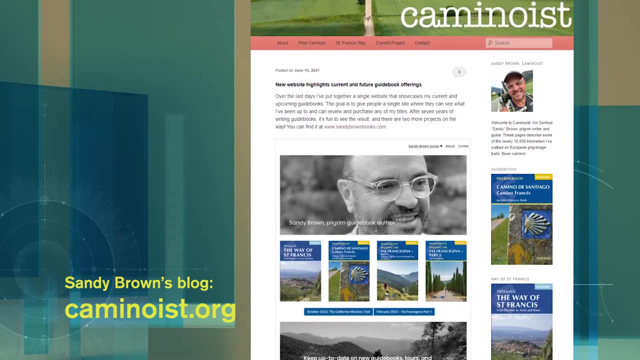 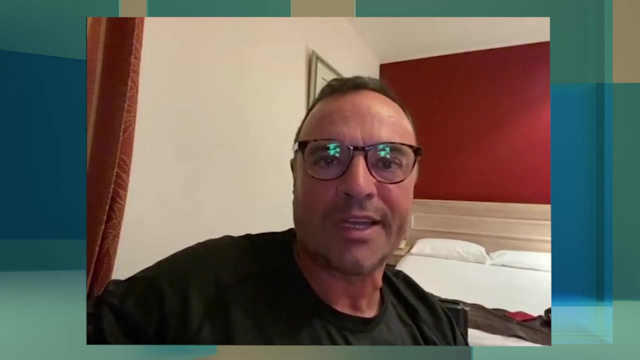 so we actually prefer that people go to the cicerone press website, which is cicerone c-i-c-e-r-o-n-e, dot, c-o, dot u-k. and cicerone, for five pounds, will send a guidebook anywhere in the world. it's going to be available to people as well, and also you can buy the guidebook as well, because amazon does such bulk buying and it forces such low prices that we make almost no money by selling a book on amazon. but you can buy it there. you can buy it on cicerone website and something to remember too is with a great publisher like ciceron press you can buy an electronic version. 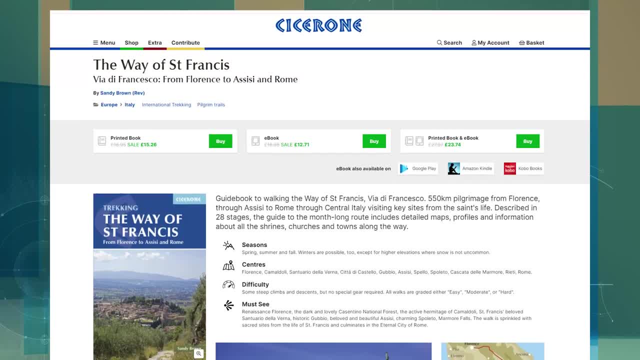 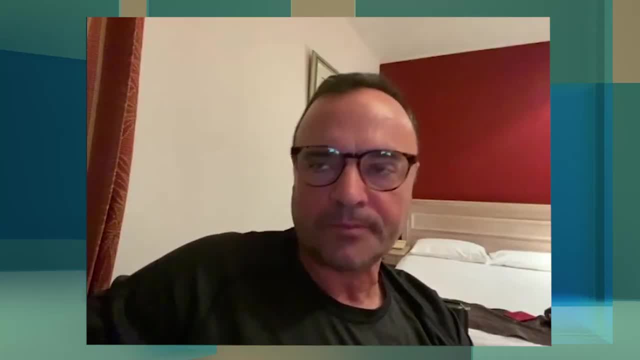 versions, including epub and kindle. and if you don't want to carry a guidebook, well, you've got your phone with you, probably, or your kindle and, um, you can have, uh, all of the information of the guidebook right there on your screen. so that's another great way to um to get that. 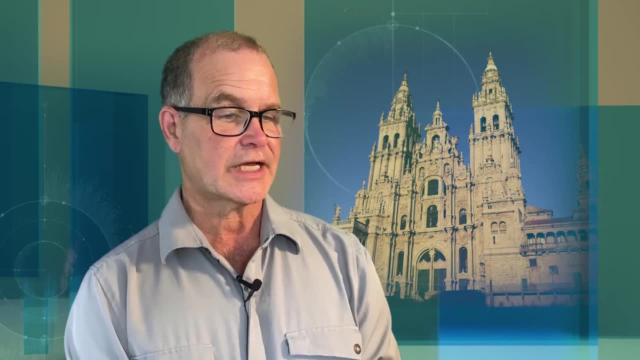 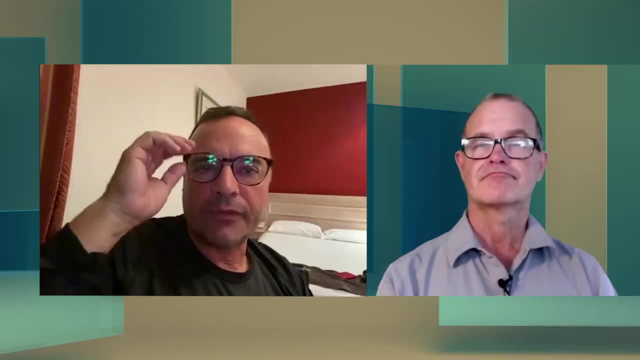 information. well, one of the last questions i always ask: is there anything else you'd like to share with the audience that i haven't asked you? yes, i want to say, if you are interested in taking a pilgrimage walk, don't be afraid, and i recommend everybody's first pilgrimage, actually.